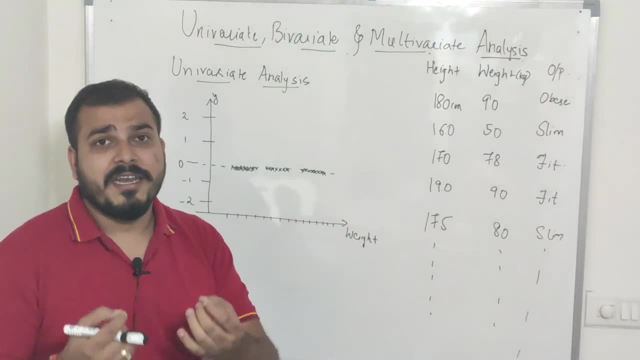 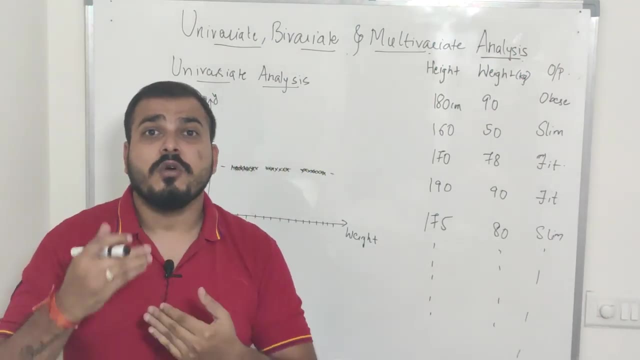 perform univariate analysis? How do we perform bivariate analysis? How do we perform multivariate analysis? Guys, remember, this is the part of the video that we're going to be talking about, part one. In the part two, I'll actually show you the practical implementation and how actually it. 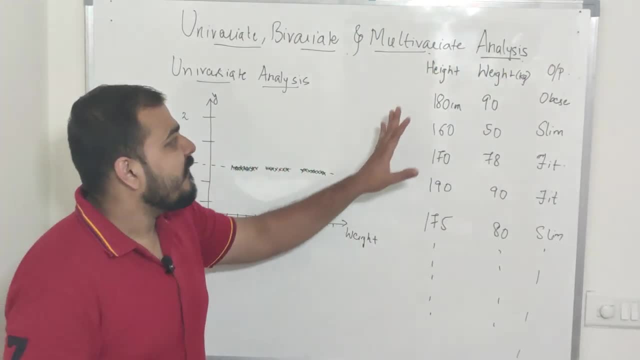 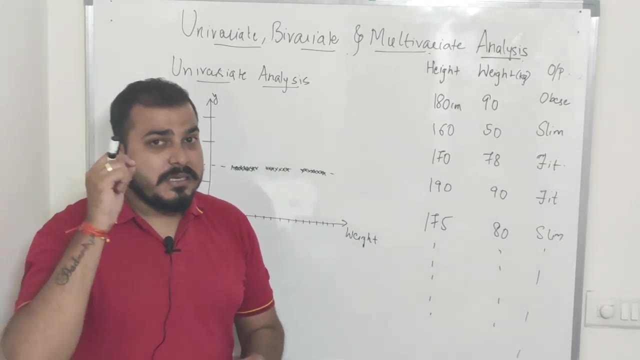 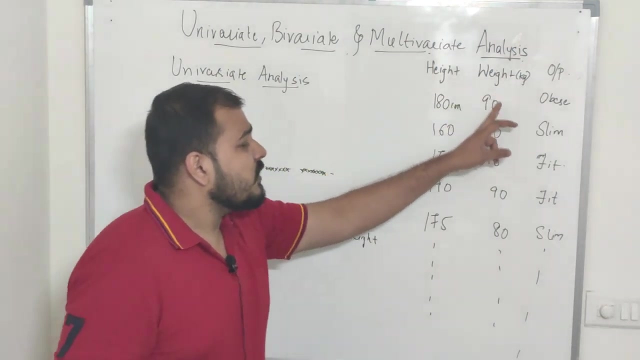 is performed. So let us go ahead. Suppose this is my data set, where I have height and weight and output. What is univariate analysis? First of all, in univariate analysis, we'll just try to pick up one feature. Okay, just we'll try to pick up one feature And, based on this feature, we will try. 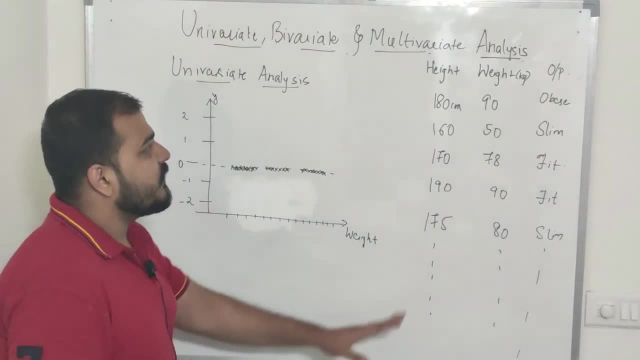 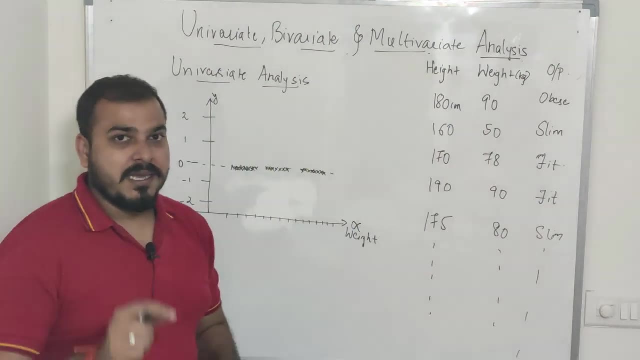 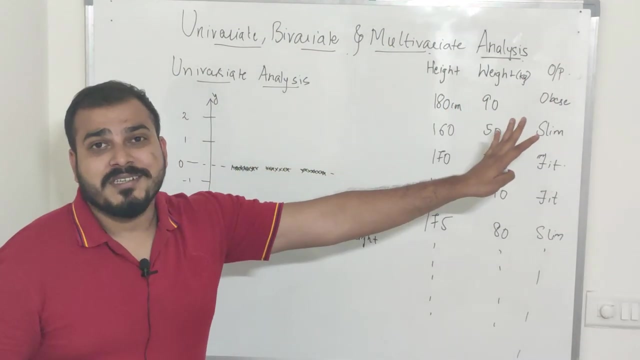 to determine what the output is. So suppose I'll take this feature as weight. Okay, I'm going to draw an x and y axis, So this is my x axis, this is my y axis, Since I am just taking only one feature, that is, weight, and I'm just trying to classify that points with respect to the output. 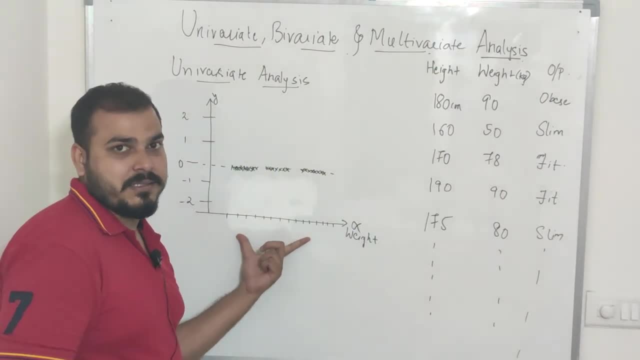 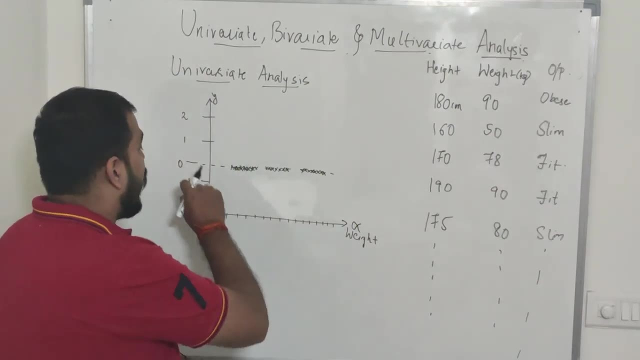 So I'm actually plotting all my weights value over here in the x axis, So in the y axis I will have nothing. Instead, I'll just try to draw a line which will be like: all the values will be zero in the y axis. So this is how it can be done. I'll show you in the part two, But make sure that you 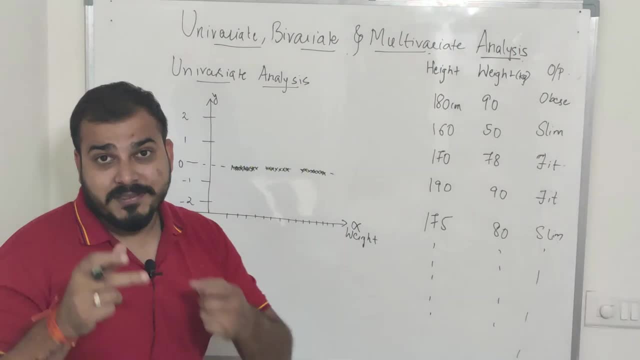 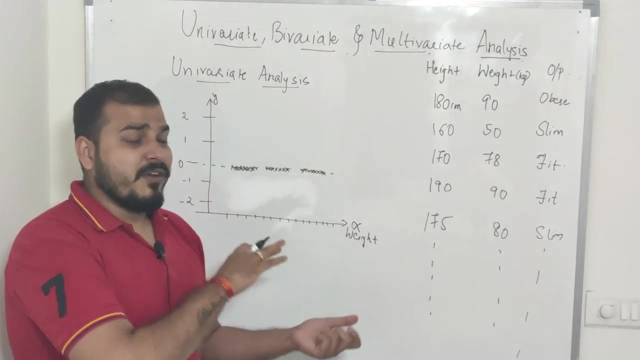 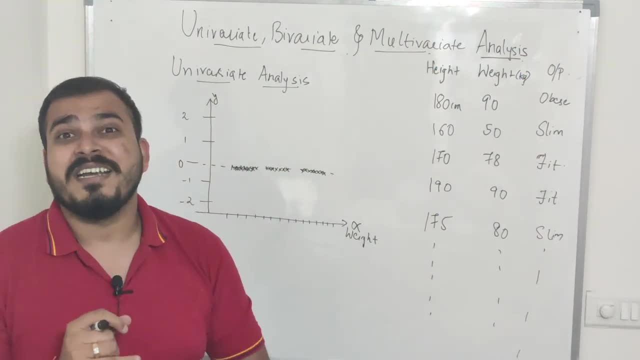 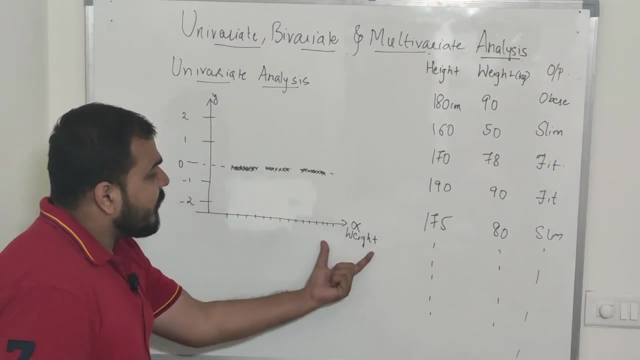 part two. we'll discuss about histogram. we'll discuss about probability density function. we'll discuss about cumulative density function, many more things. So over here I'm just plotting with respect to this: weights, what are the values? So these are the values. I'm actually trying to 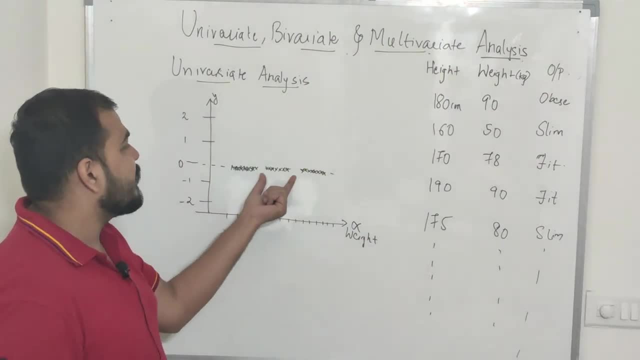 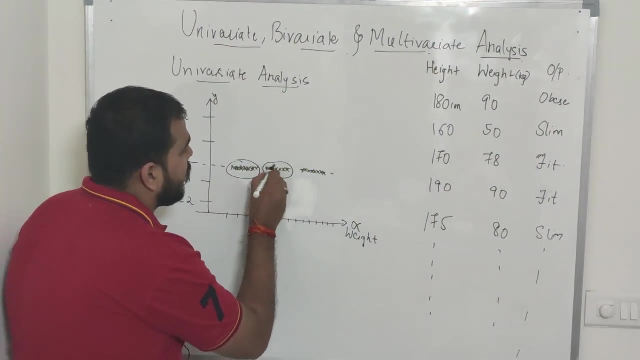 plot And over here you can see that these values are basically slim, these values are basically fit And these values are basically my obese category. So over here I can basically see three categories. Okay Now, by this, considering weight, are we able to classify the points? Yes, 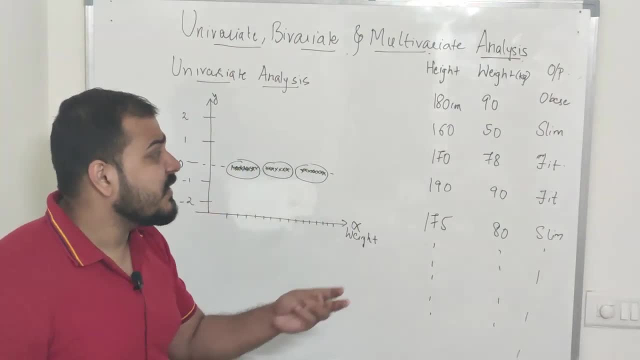 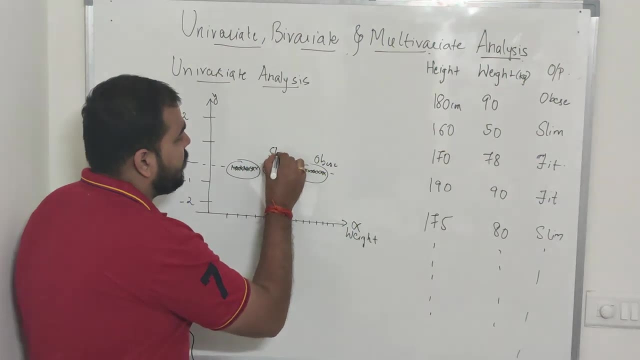 we are able to classify the points or classify the three categories- that is, obese, slim and fit- very, very easily. So this is my obese category. This is my slim- sorry, fit category. And this is my slim category. So let's just let me rub it. So this is my fit category. 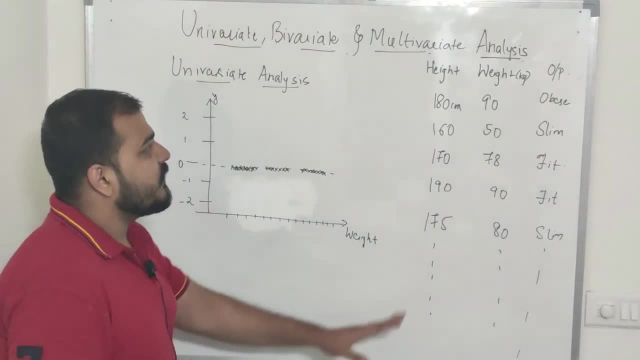 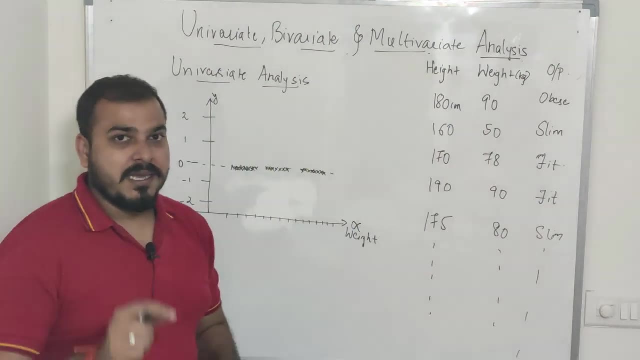 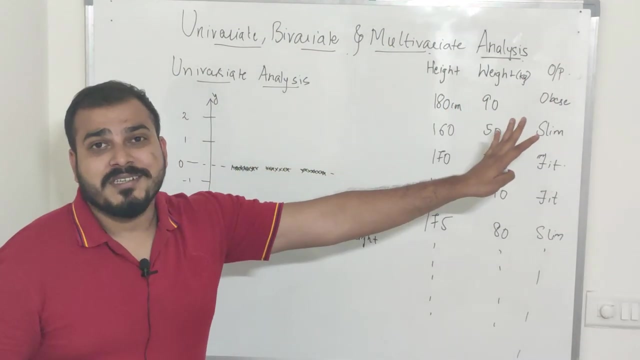 to determine what the output is. So suppose I'll take this feature as weight. Okay, I'm going to draw an x and y axis, So this is my x axis, this is my y axis, Since I am just taking only one feature, that is, weight, and I'm just trying to classify that points with respect to the output. 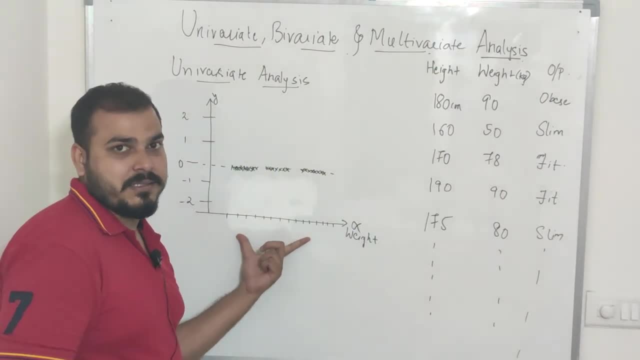 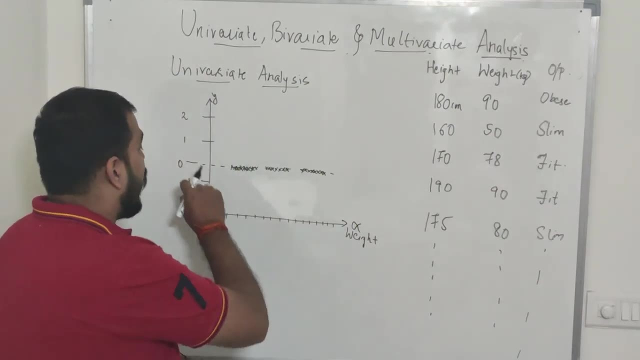 So I'm actually plotting all my weights value over here in the x axis, So in the y axis I will have nothing. Instead, I'll just try to draw a line which will be like: all the values will be zero in the y axis. So this is how it can be done. I'll show you in the part two, But make sure that you 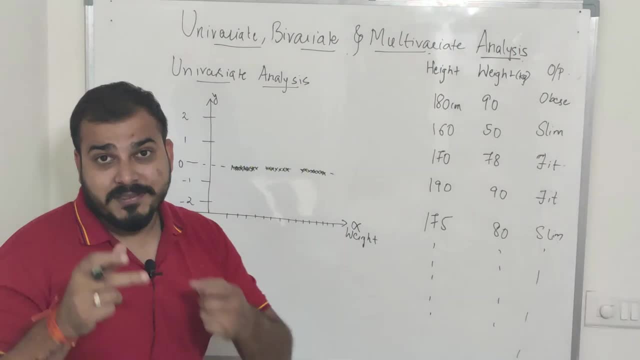 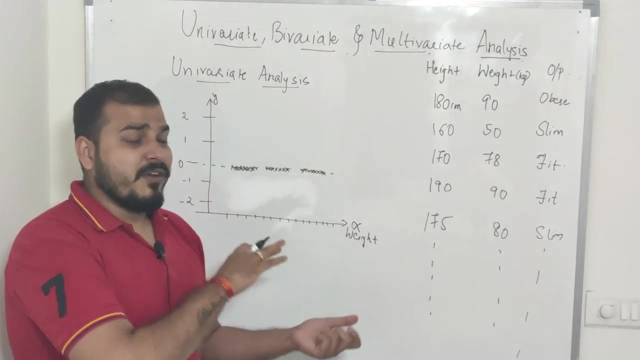 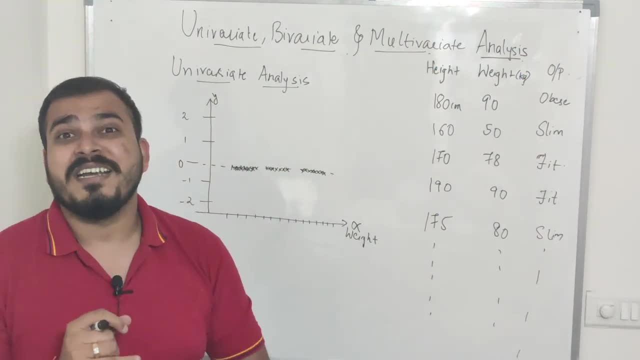 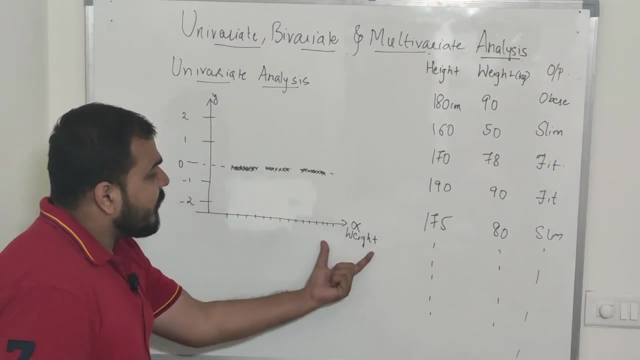 part two. we'll discuss about histogram. we'll discuss about probability density function. we'll discuss about cumulative density function, many more things. So over here I'm just plotting with respect to this: weights, what are the values? So these are the values. I'm actually trying to 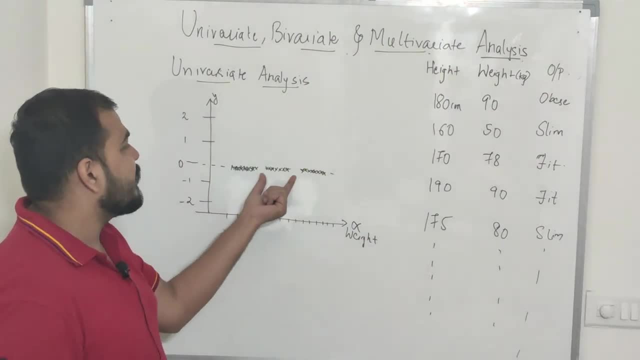 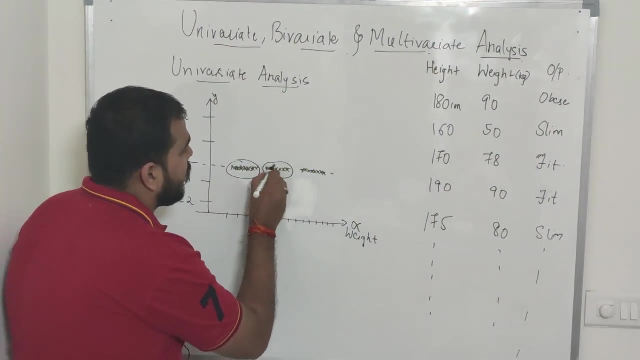 plot And over here you can see that these values are basically slim, these values are basically fit And these values are basically my obese category. So over here I can basically see three categories. Okay Now, by this, considering weight, are we able to classify the points? Yes, 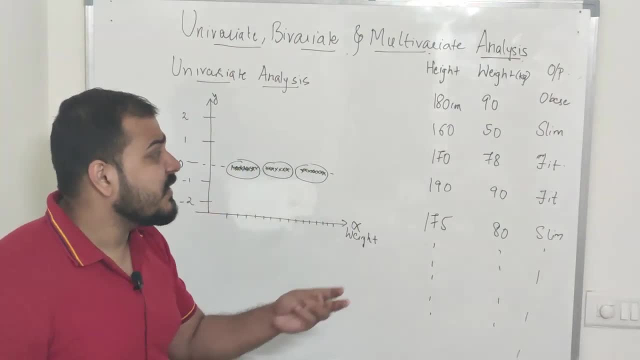 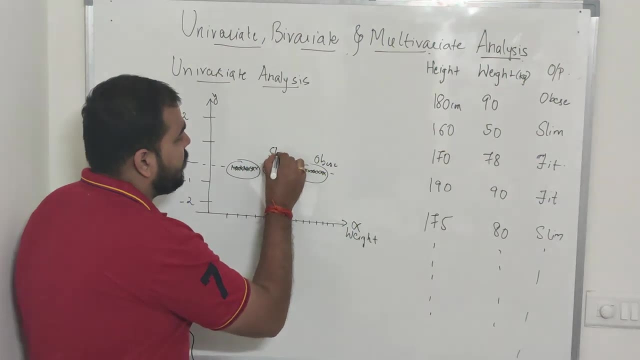 we are able to classify the points or classify the three categories- that is, obese, slim and fit- very, very easily. So this is my obese category. This is my slim- sorry, fit category. And this is my slim category. So let's just let me rub it. So this is my fit category. 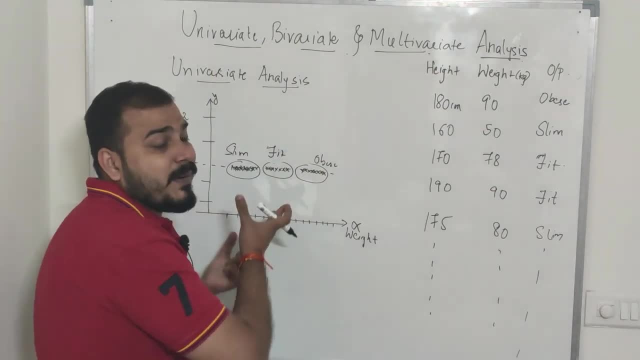 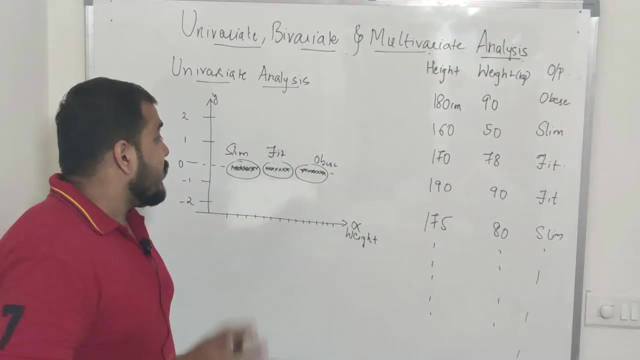 Now, what do you see from this particular- you know this particular graph over here. you can basically see that just with the help of weight I'm able to classify the output. Now you should also understand guys like this kind of points will not be always there. you will not be easily. 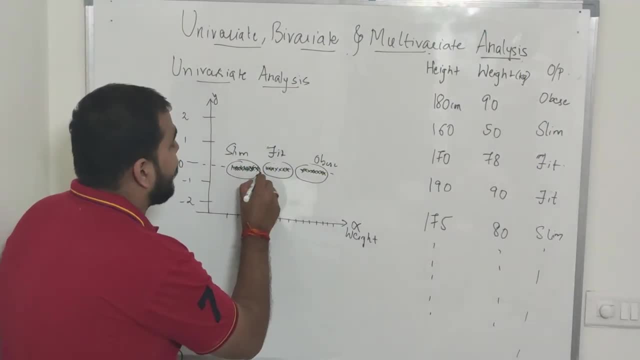 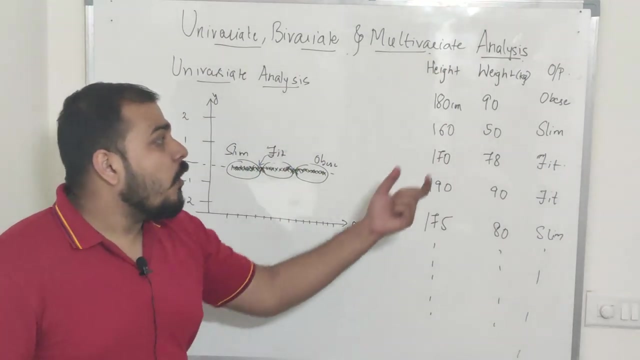 able to classify all the points. some of the points may also be overlapping, So this may be my fit category like this. you know, suppose the obese is also overlap, So a lot of points will be there and I will not be able to classify the output categories correctly. So, due to that, what we do, 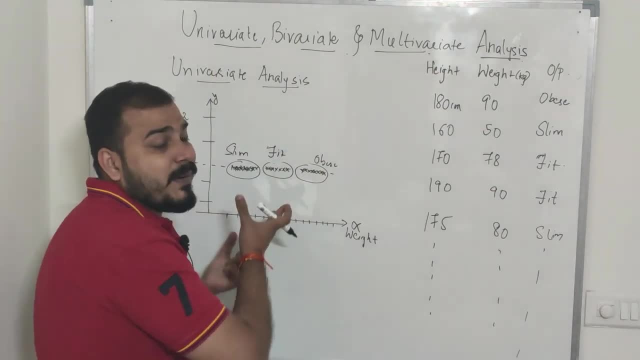 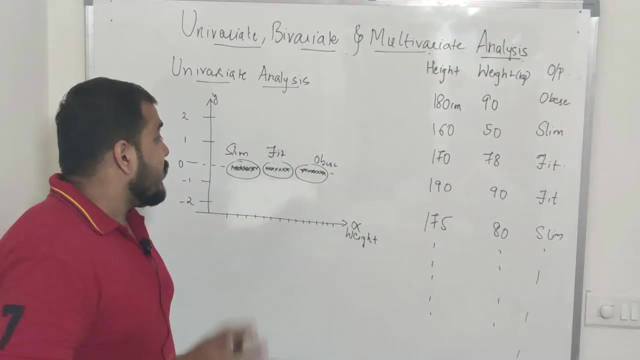 Now, what do you see from this particular- you know this particular graph over here. you can basically see that just with the help of weight I'm able to classify the output. Now you should also understand guys like this kind of points will not be always there. you will not be easily. 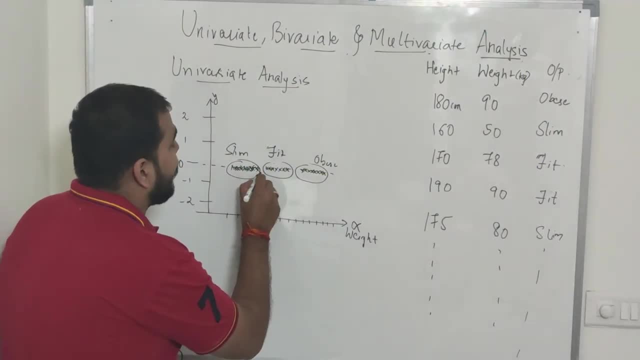 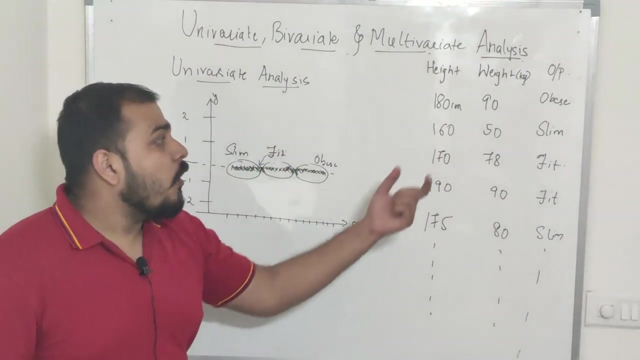 able to classify all the points. some of the points may also be overlapping, So this may be my fit category like this. you know, suppose the obese is also overlap, So a lot of points will be there. but just by using one feature I will not be able to classify the output categories correctly. So due. 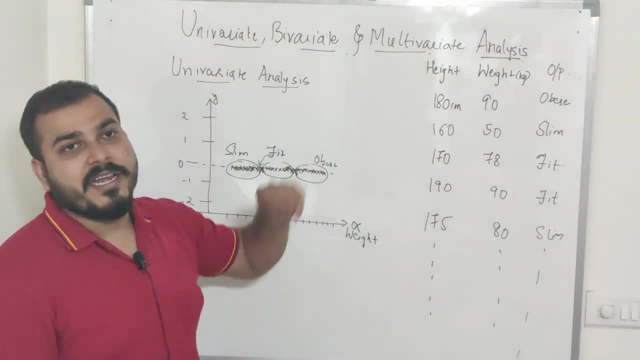 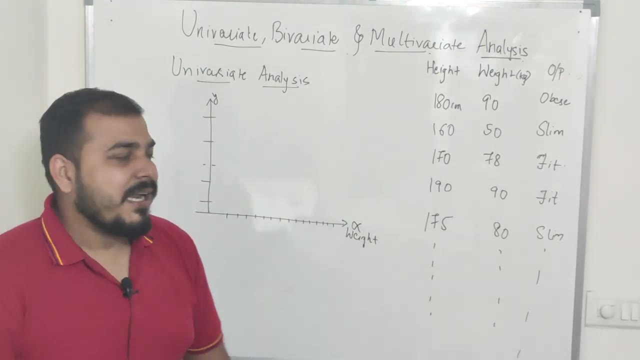 to that. what we do is that we go with the bivariate analysis and multivariate analysis. So let us go ahead and try to understand what exactly is bivariate analysis. So in bivariate analysis we'll be taking at least two features like height and weight. So suppose in my y axis I have height. 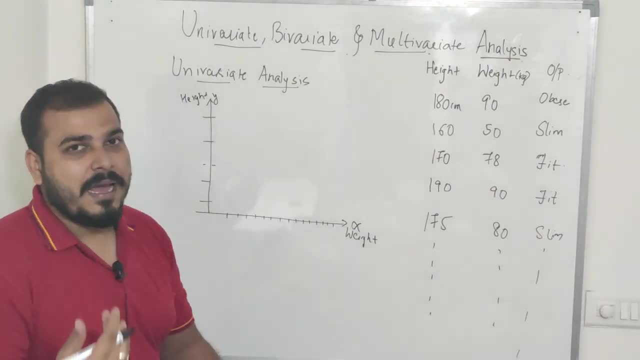 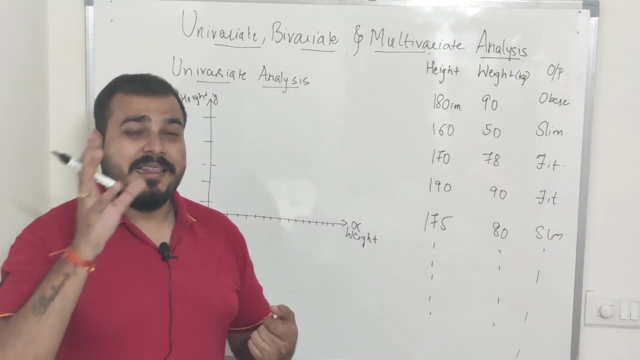 and in the x axis I have weight. Okay, now, usually what happens is that in most of the scenario, as the weight also increases- because this is what we get from the domain knowledge right, And they are some outliers where people with less height will be actually obese- they'll be having more. 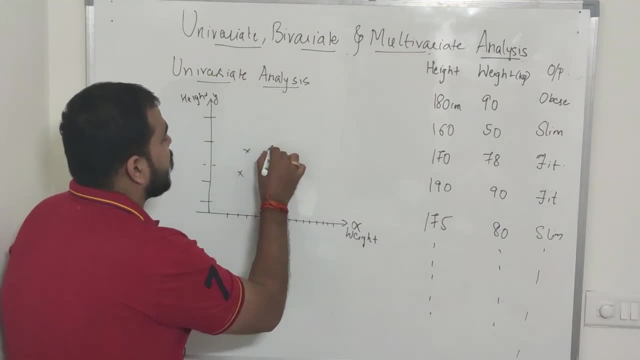 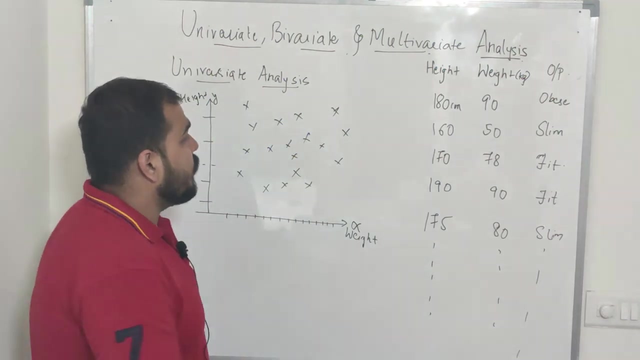 weight. So some of the points will be plotted somewhere like this: you know, and this is how this particular points will be plotted most of the time. Okay, so these are my points Now, based on this particular points. again, if I try to see the outputs, I will be able to classify this particular. 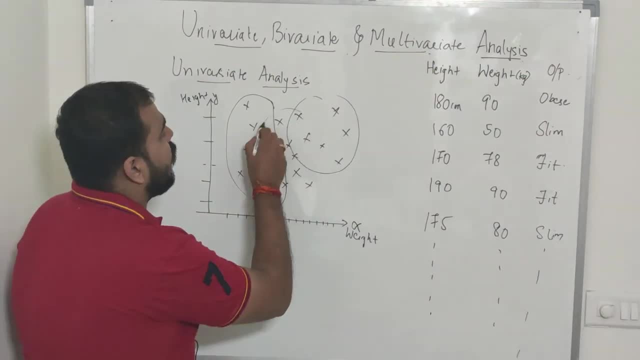 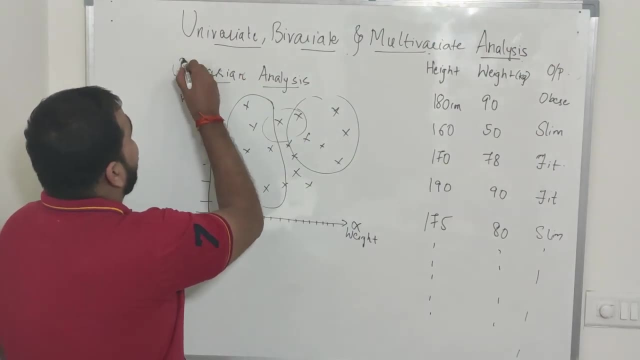 points Somewhere like this. okay, and some of the points will also be overlapped. So here this is basically my bivariate analysis, So let me just write it down over here as bivariate analysis. In bivariate analysis, we are actually trying to see two features, And then we are trying to see how the 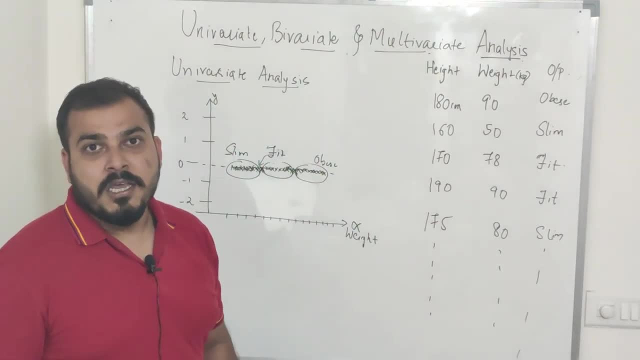 is that we go with the bivariate analysis and multivariate analysis. So let us go ahead and try to understand what exactly is bivariate analysis. So in bivariate analysis we'll be taking at least two features like height and weight. So suppose in my y axis I have height and in the x axis 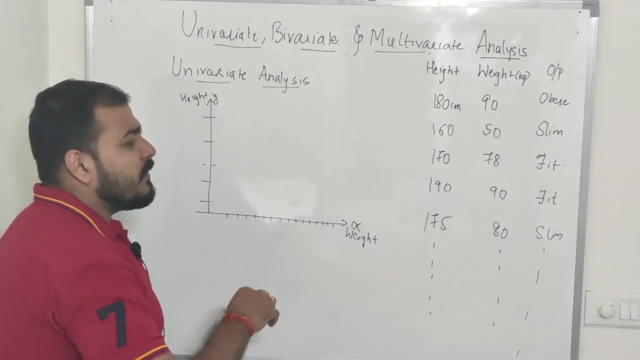 I have weight. Okay, Now, usually what happens is that in most of the scenario, as the height increases, the weight also increases, because this is what we get from the domain knowledge right, And they are some outliers where people with less height will be actually obese: they'll be having more. 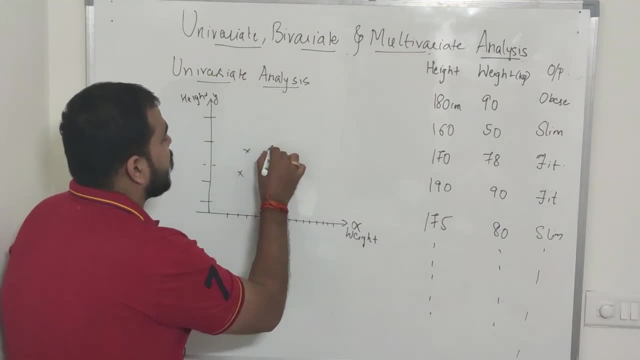 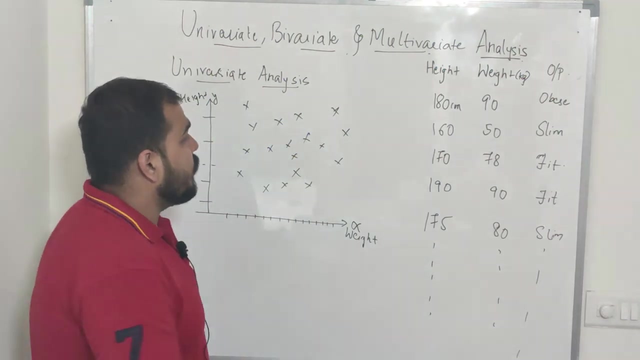 weight. So some of the points will be plotted somewhere like this: you know, and this is how this particular points will be plotted most of the time. Okay, so these are my points Now, based on this particular points. again, if I try to see the outputs, I will be able to classify this particular. 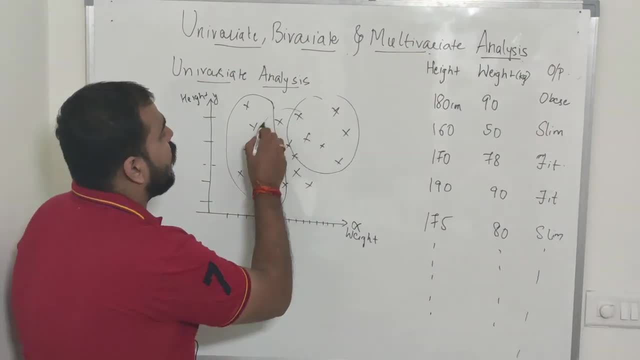 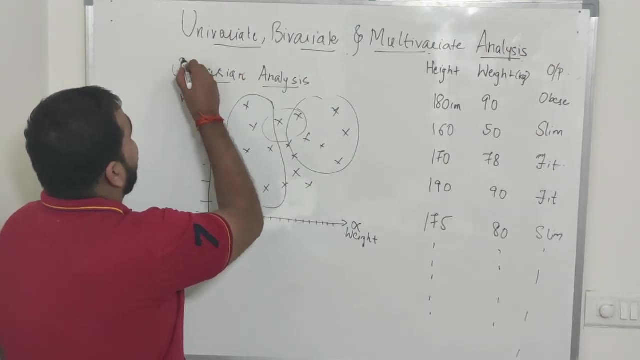 points Somewhere like this. okay, and some of the points will also be overlapped. So here this is basically my bivariate analysis, So let me just write it down over here as bivariate analysis. In bivariate analysis, we are actually trying to see two features, And then we are trying to see how the 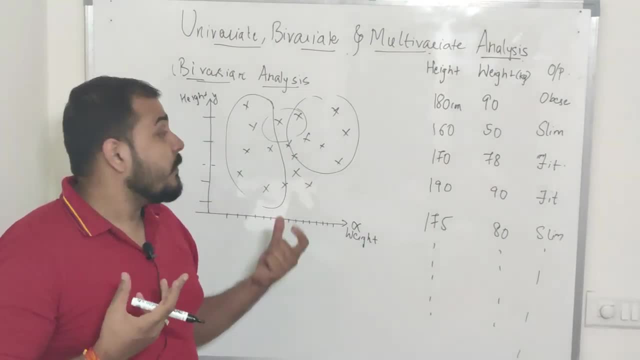 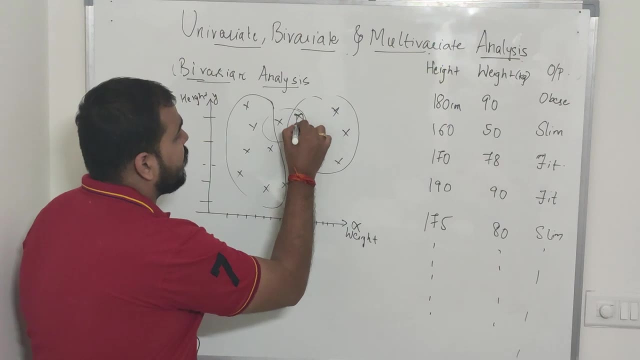 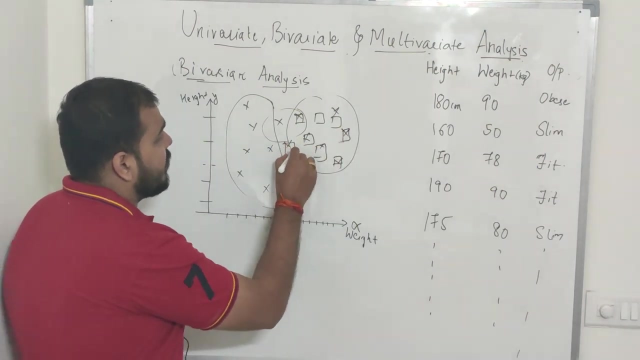 output is basically done And a lot of things can. you can come from this particular graph also. guys understand that. suppose I have two different classes over here. Suppose this is one of my class, Okay, Okay, And this cross is basically one of my class, Okay, And you will be able to see that some of the points will be. 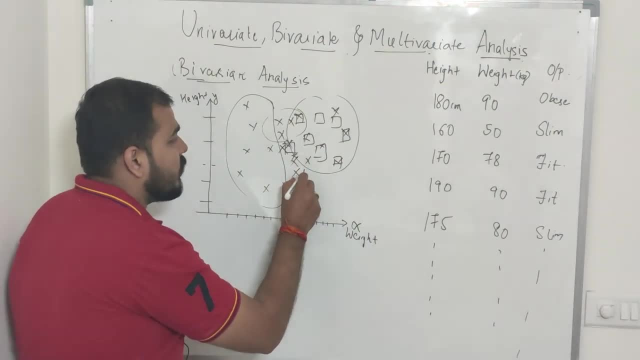 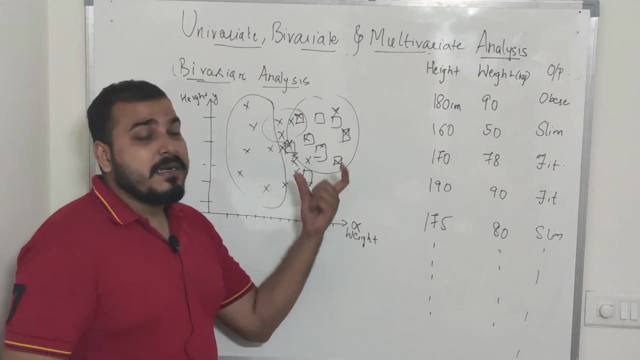 overlapping, Okay, And when the points are overlapped, this will also help you to understand that. which machine learning algorithm should I try to apply? Now? this is very important, guys. If we are able to classify the points properly, I can definitely use a logistic regression. right, I can definitely use a logistic. 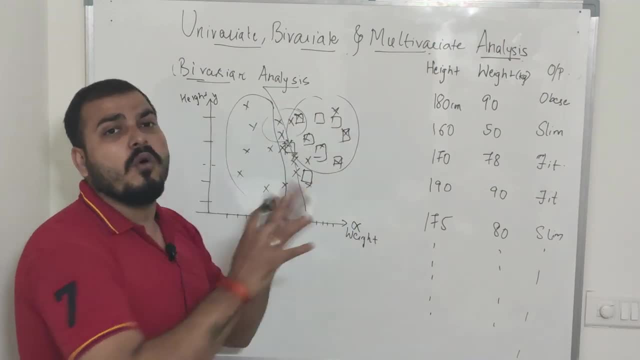 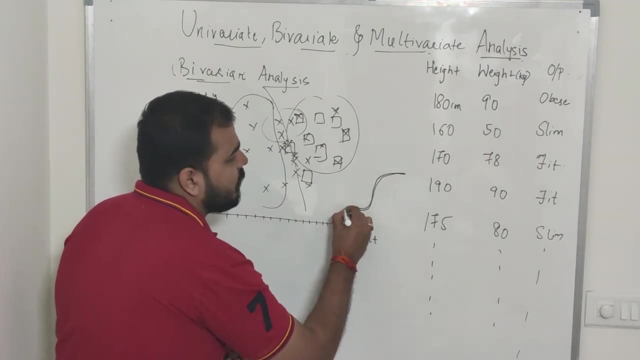 regression and try to classify these points, But if they are so much of overlapping of the points, definitely I cannot use logistic regression. Logistic regression uses a concept of sigmoid right, So here this particular line will help us to classify. but this is. 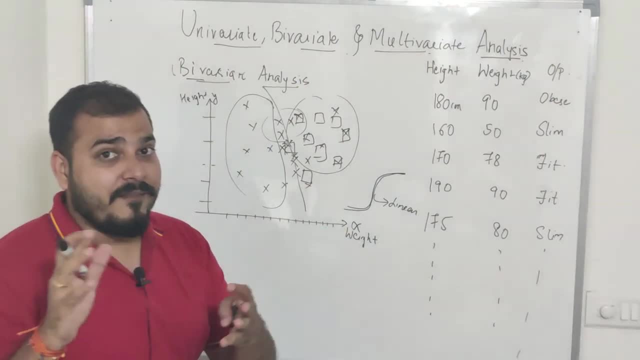 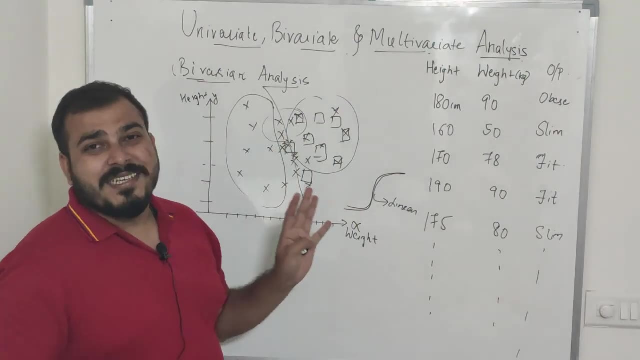 basically a linear line. I know you will be having confusion. in logistic regression we actually draw a linear line and try to divide the points right. So if my points are not easily divided, I will definitely not go with logistic regression, because I 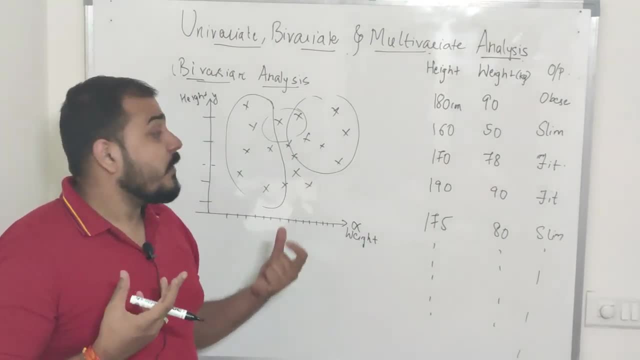 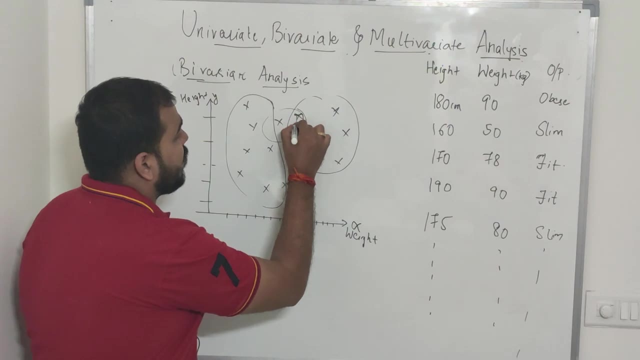 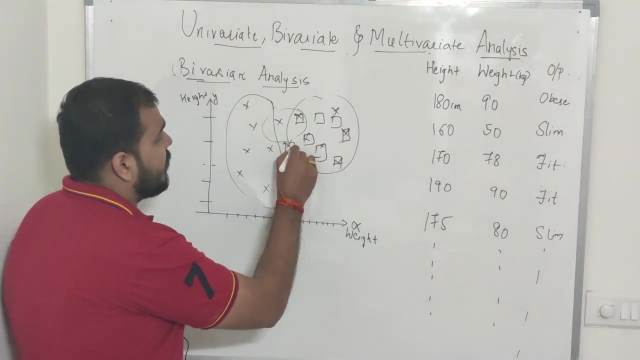 output is basically done And lot of things can. you can come from this particular graph also. guys understand that suppose I have two, two different, different classes over here. Suppose this is one of my class, okay, Okay, And this cross is basically one of my class, Okay, And you will be able to see that some of the 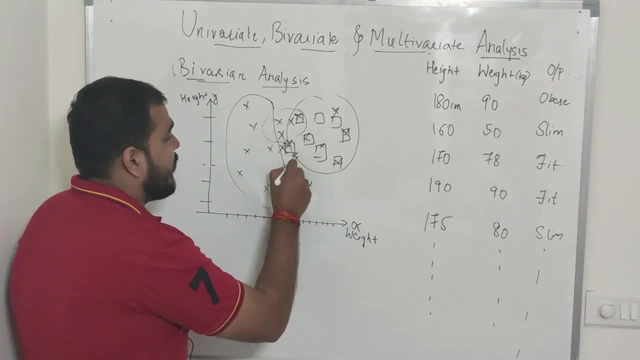 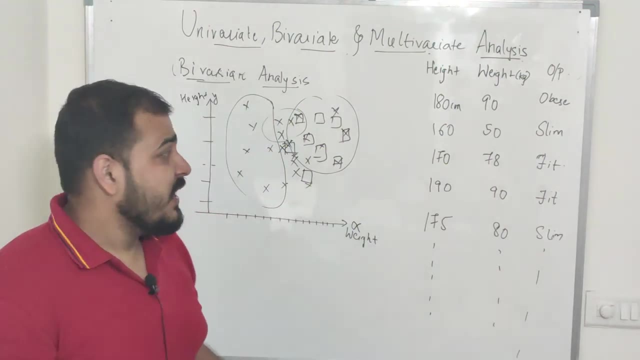 points will be overlapping, Okay, And when the points are overlap, this will also help you to understand that. which machine learning algorithm should I try to apply Now? this is very important, guys. if we are able to classify the points properly, I can definitely use a logistic. 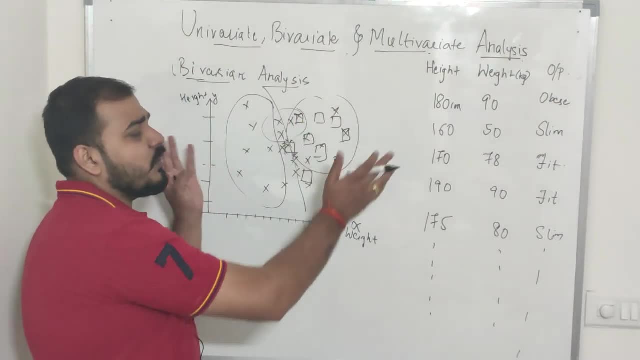 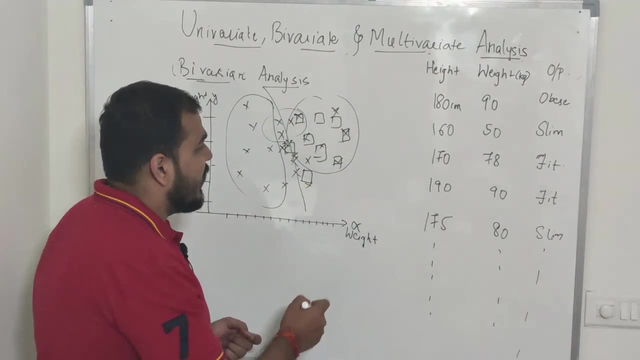 regression right. I can definitely use a logistic regression and try to classify this points, But if they are so much of overlapping of the points, definitely I cannot use logistic regression because lot of our points are overlapping. logistic regression uses a concept of sigmoid, right. so here this particular line will help. 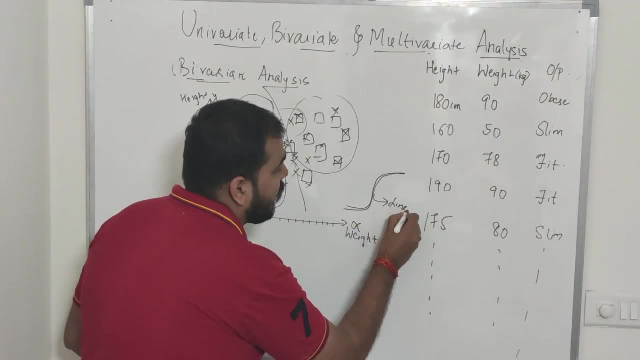 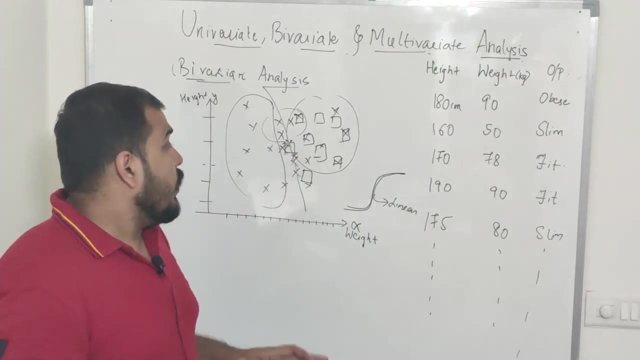 us to classify, but this is basically a linear line. i know you will be having confusion. in logistic regression we actually draw a linear line and try to divide the points right. so if my points are not easily divided, i will definitely not go with logistic regression, because i will be. 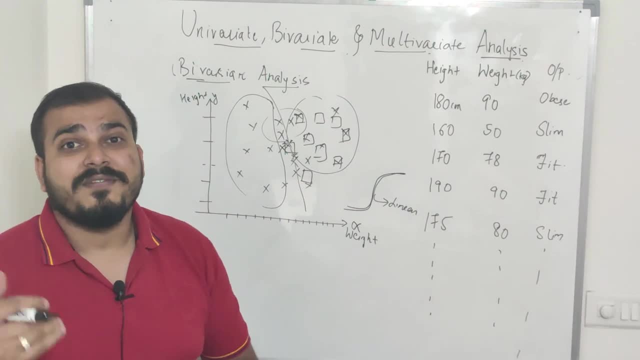 getting high errors. that time i'll be going with non-linear classifying problems like decision trees, like random forest, like xg boost or like svm, like and again advanced concepts of our ada boost. so all those kind of algorithm i can basically choose in order to solve if there is. 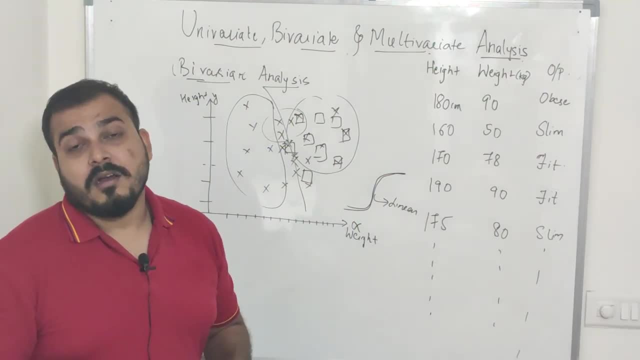 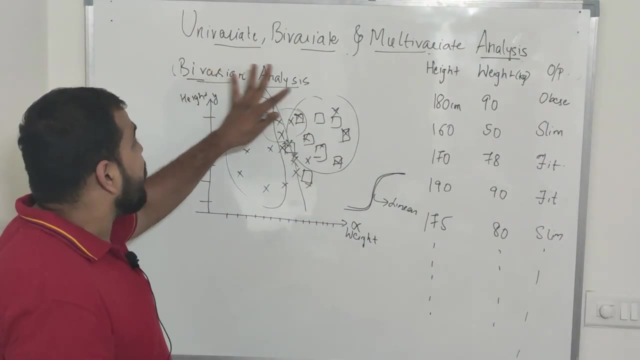 so much of overlapping. okay, i can also use knn algorithms so i can verify this particular thing by just seeing this particular graph very, very easily. right, and that is what bivariate analysis basically says. but what will happen if i have more features over here, if i have four features? 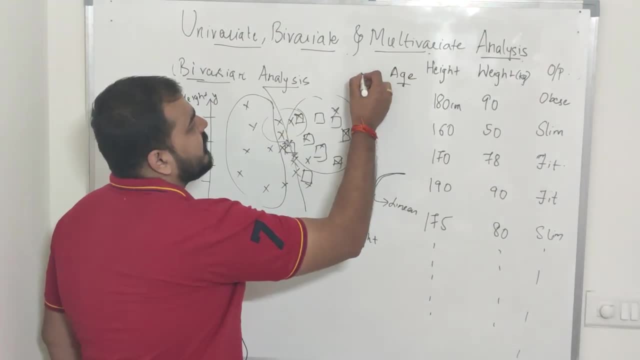 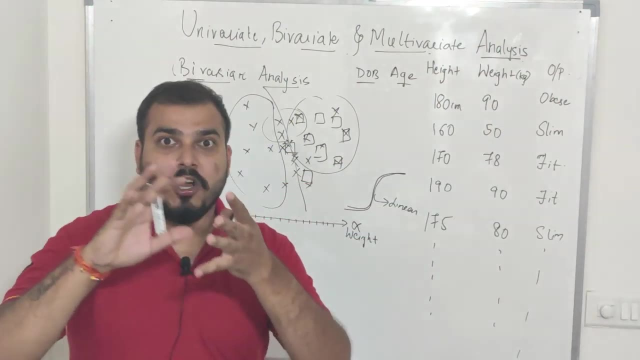 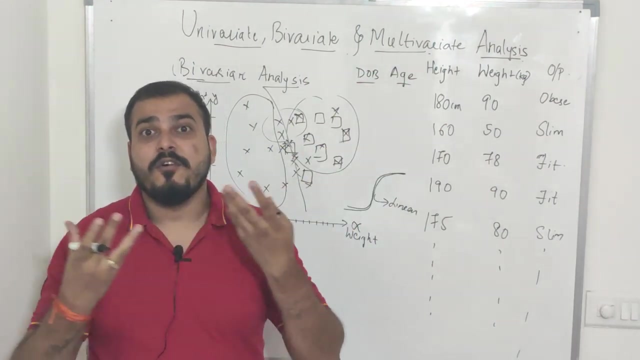 suppose this is my age. this is my third feature. suppose i'll say that this is my date of birth. i'm just considering some examples. i'm adding some features. right, if i have three features, i can draw a 3d diagram. okay, i can draw a 3d diagram. but if i have four features, you can. no one can see actually a 4d diagram- we human being. 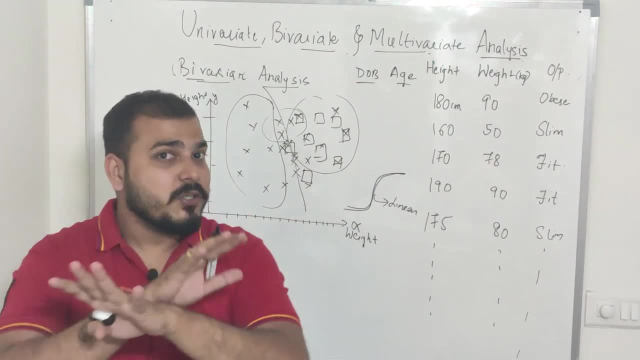 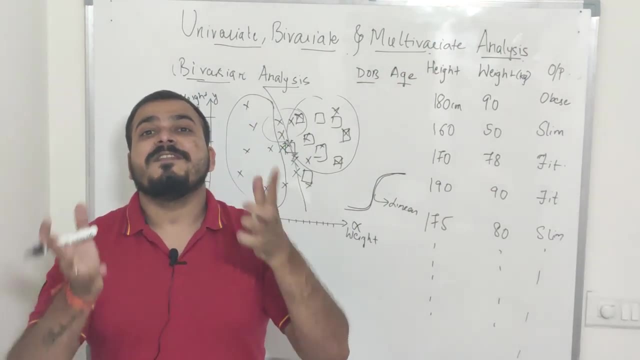 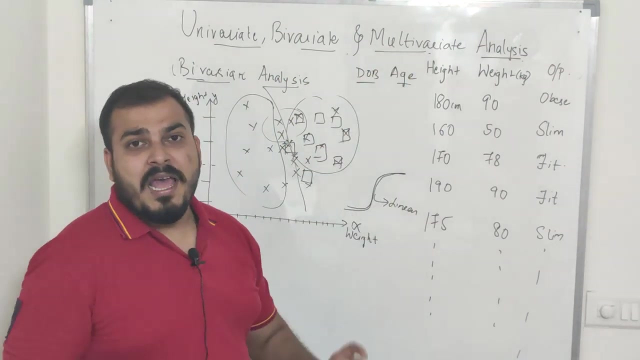 definitely it is not possible in this particular life. you know you should. you cannot actually see a 4d diagram. so, in order to solve this particular 4d diagram- how do you see the features at that time- we will basically be using the multivariate analysis. now how the multivariate analysis is done. 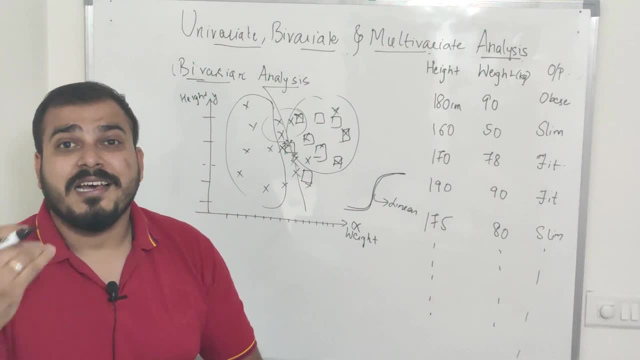 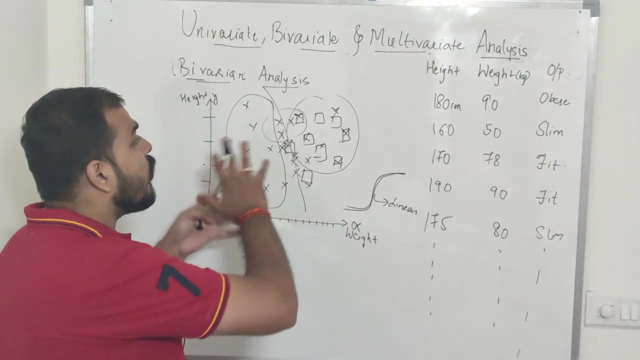 will be getting high errors. That time I'll be going with nonlinear classifying problems like decision trees, like random forest, like XGBoost, Like SVM, like, and again, advanced concepts of Jahrida, boost, So all those kind of algorithms I can basically choose in order to solve if there is so much of overlapping. 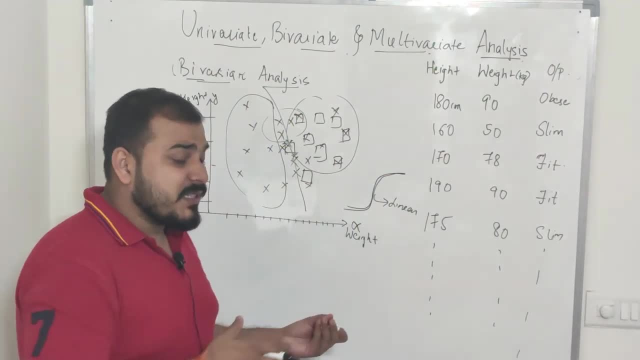 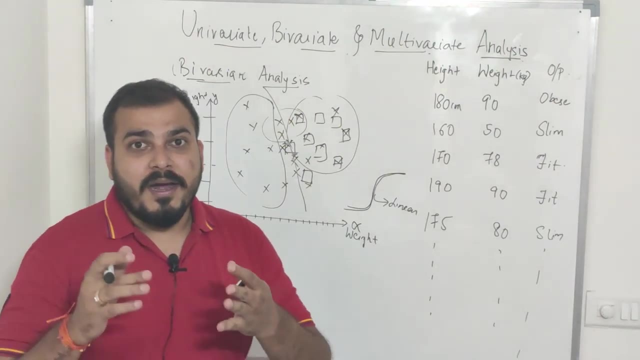 Okay, I can also use KNN algorithms, So I can verify this particular thing by just seeing this particular graph very, very easily. right, And that is what bivariate analysis basically says. But what will happen if I have more features over here, if I have four features? suppose this is my age? this is my third feature. 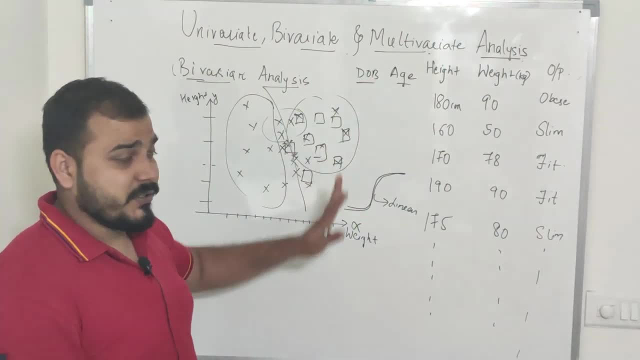 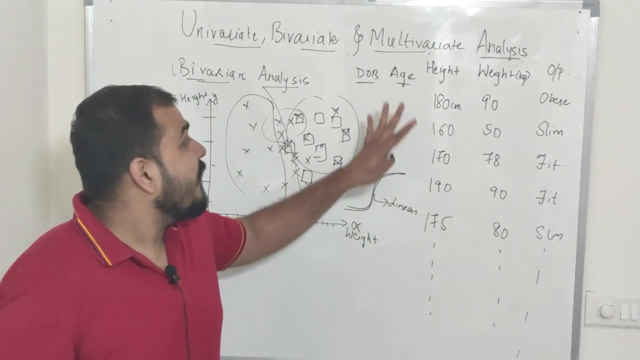 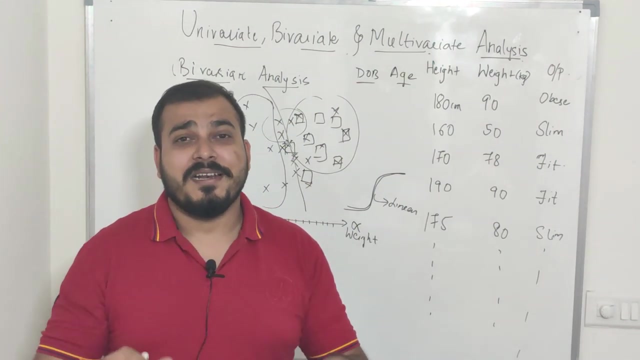 is my date of birth. i'm just considering some examples and adding some features. right, if i have three features i can draw a 3d diagram. okay, i can draw a 3d diagram, but if i have four features, you can. no one can see actually a 4d diagram- we human being definitely. it is not possible in this. 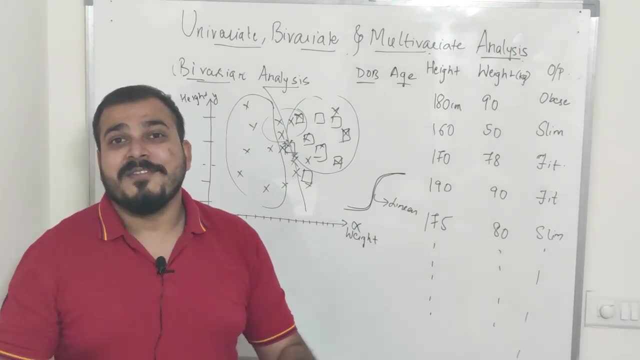 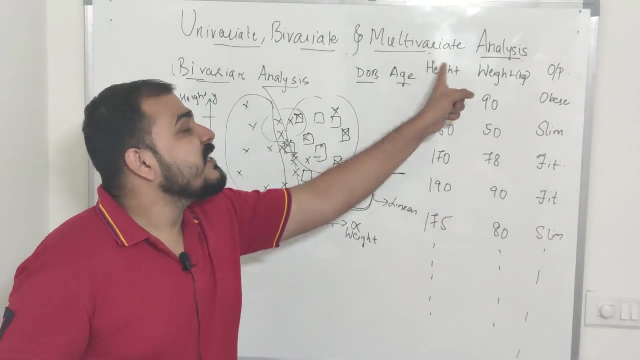 particular, you know you should, you cannot actually see a 4d diagram. so in order to solve this particular 4d diagram- how do you see the features at that time, we will basically be using the multivariate analysis. now, how the multivariate analysis is done, i'll just draw a diagram over. 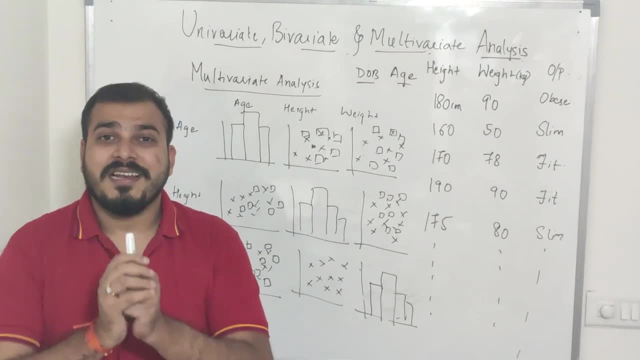 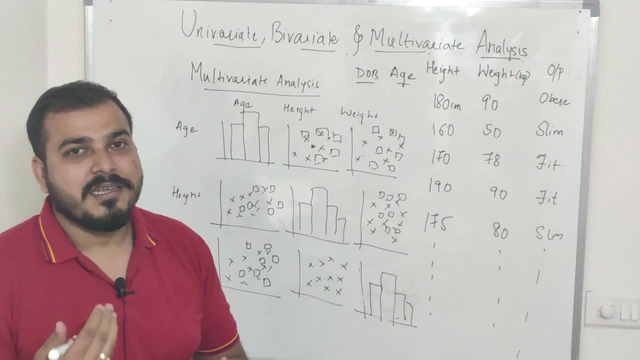 here and i'll try to show you. show it to you, okay. so, guys, let us go ahead and try to understand. how does a multivariate analysis work? and this is basically the diagram. understand, guys? if you have more than three and four features, at that time you cannot basically see a 4d diagram here. 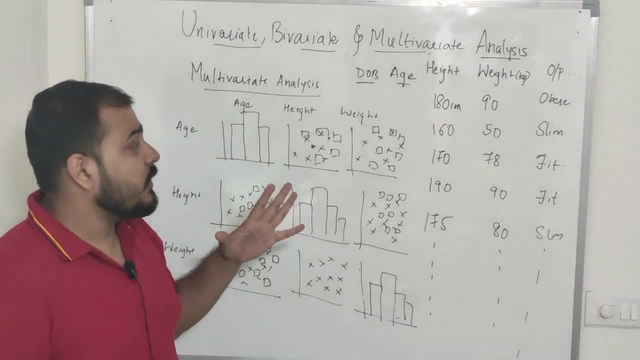 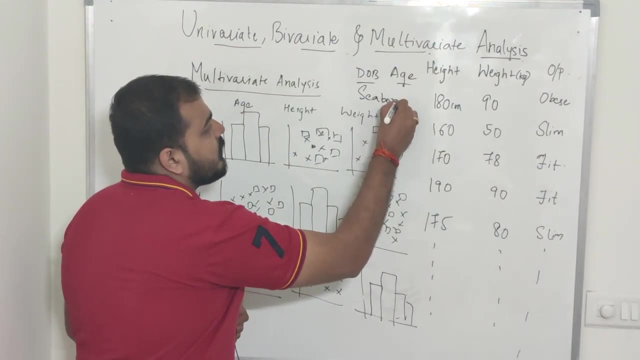 again, i've taken an example of three features. uh, here in the uh, if i just consider about multivariate analysis, there's a very good library which is called a seaborn, which will help us to do that. you know, seaborn has a function which is called as pair plot. with the help of pair plot, you will 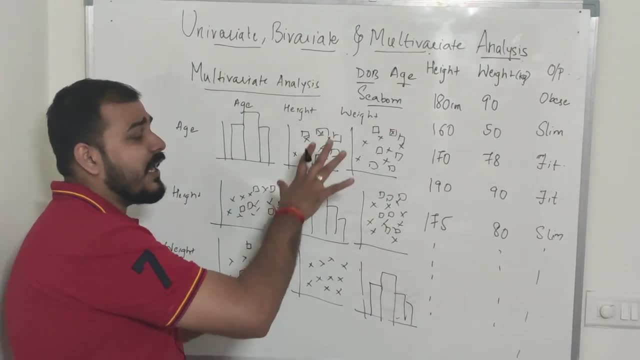 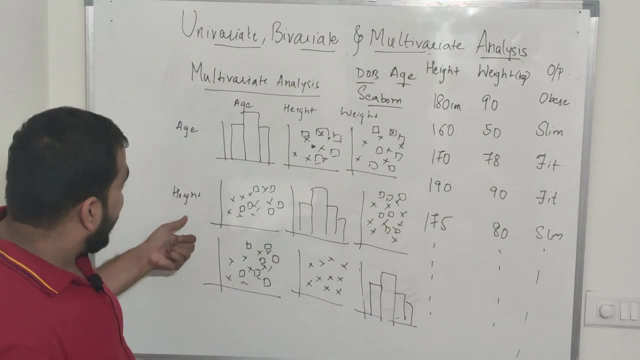 be able to see this particular analysis and how the values are actually plotted. so how does a multivariate analysis actually work? so in the x-axis, in the y-axis, you can see that i have features: age, height and weight- okay, and in this particular x-axis also, i have age, height and 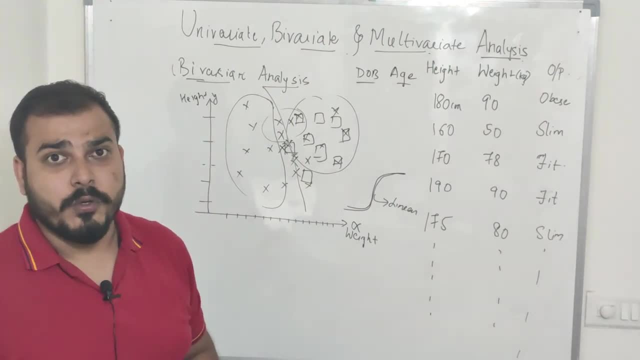 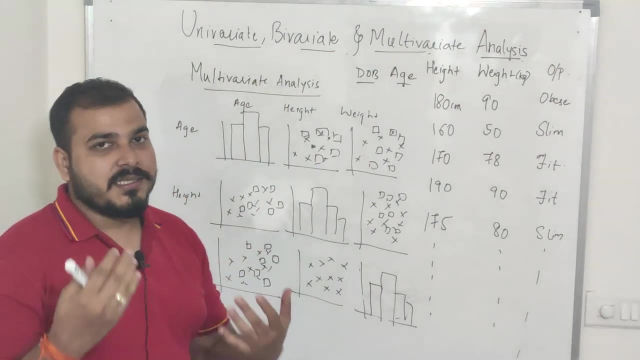 i'll just draw a diagram over here and i'll try to show you. show it to you, okay. so, guys, let us go ahead and try to understand. how does the multivariate analysis work? and this is basically the diagram. understand, guys? if you have more than three and four features, at that time you cannot. 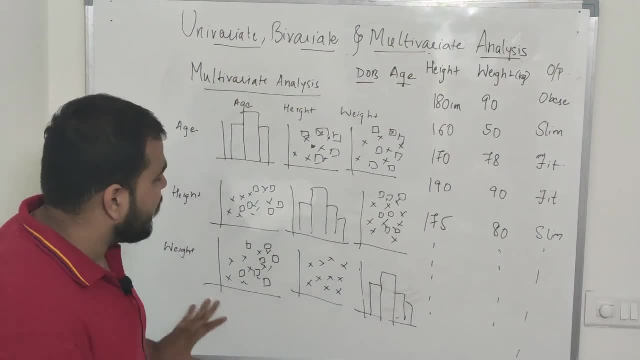 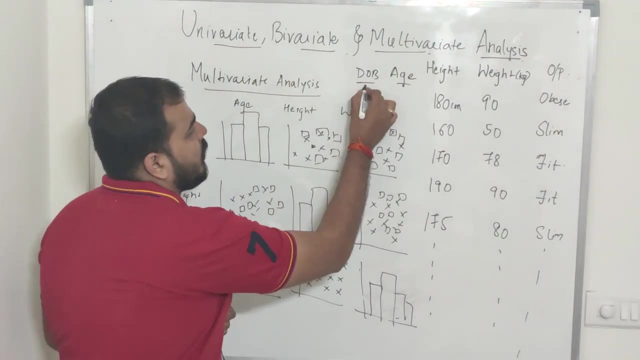 basically see a 4d diagram. here again, i've taken an example of three features. uh, here in the uh, if i just consider about multivariate analysis, there's a very good library which is called a seaborn which will help us to do that. you know, seaborn has a function which is called as pair. 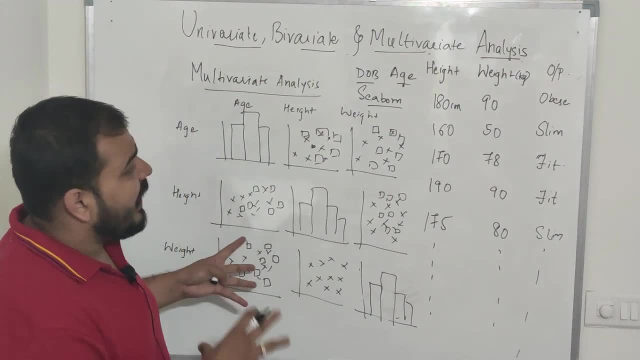 plot. with the help of pair plot, you will be able to see this particular analysis and how the values are actually plotted. so how does a multivariate analysis actually work? so in the x-axis, in the y-axis, you can see that i have features: age, height and weight, okay, and in this particular x-axis also. 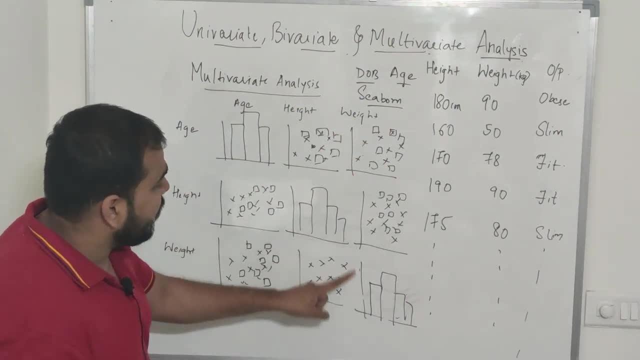 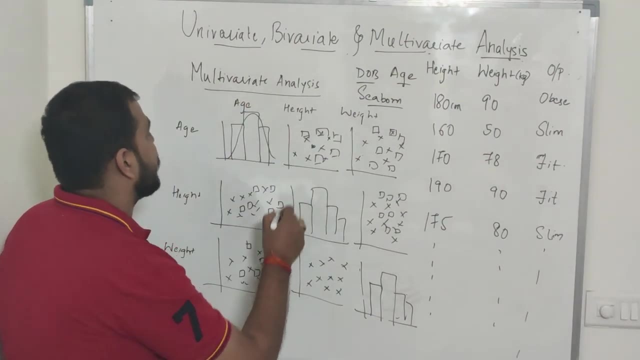 i have age, height and weight. now what will happen is that this diagrams that will get plotted will be compared to this feature and this feature suppose, if i see age and age, definitely at that time i'll be getting a histogram with some probability density function. i'll just again: 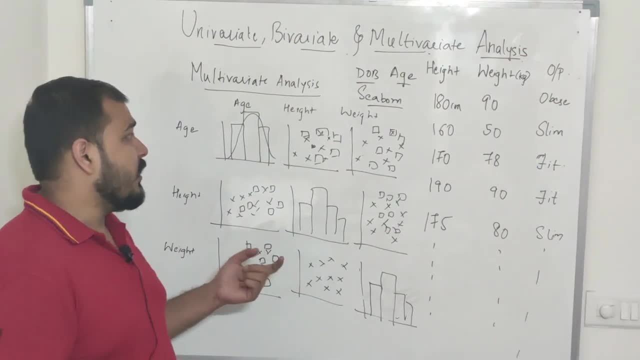 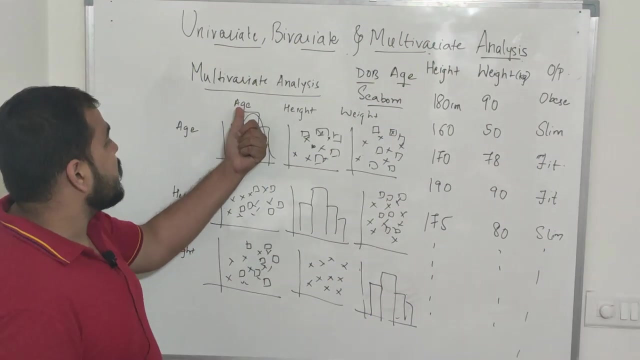 don't worry about histogram right now. in my upcoming classes, i'll be explaining you about that now. this particular diagram that i see is between age and height and based on that that particular points are basically highlighted. similarly, this age and weight- you can see this points are getting highlighted in my next row when i go. this is basically my height and this is. 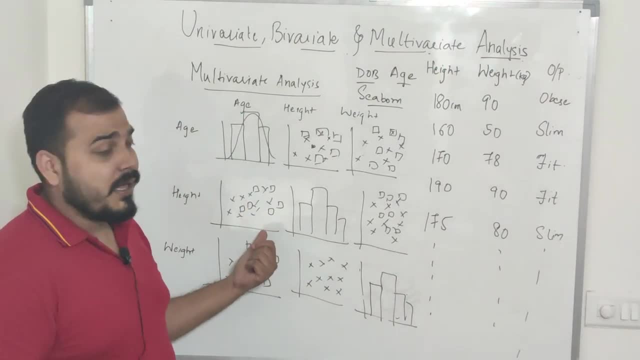 basically my age. now i can see that how this particular points has been plotted. all these points are getting highlighted. so this is basically my height and this is basically my age. all this will be explained in the part 2 and i'll be showing you practically how it we can basically. 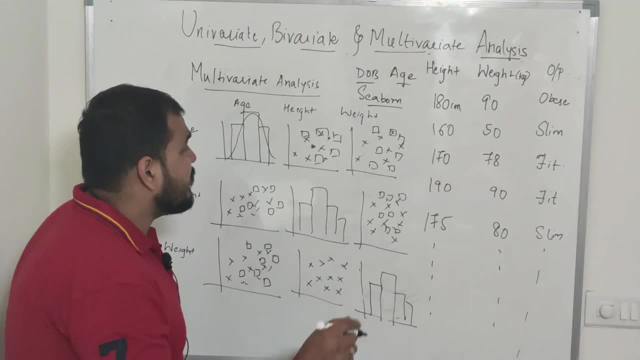 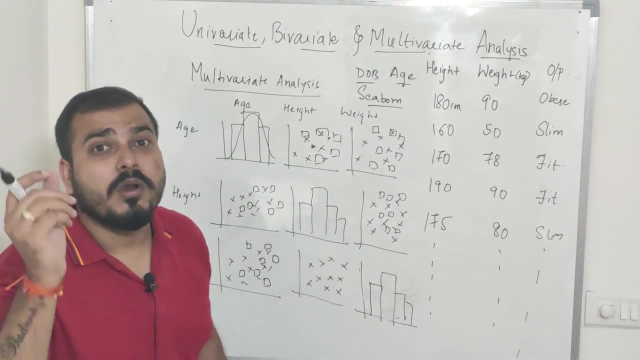 do, with the help of seaborn, with a perfect example. now understand these things, guys. this diagrams, right? these diagrams can also lead to something called as correlation. you will get an idea of correlation. what does correlation basically mean? if you have not seen my videos in statistics, i've 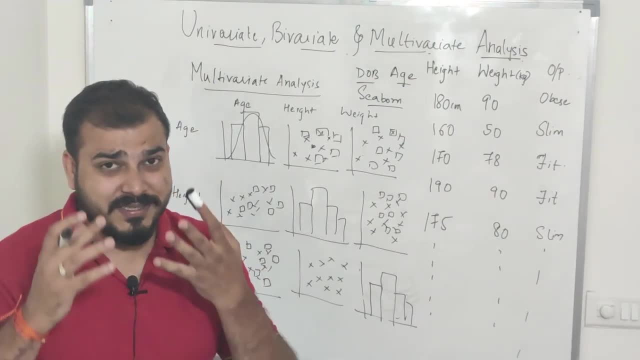 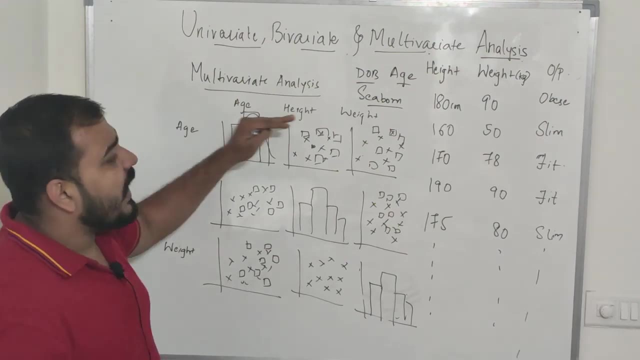 actually created a video on covariance pearson correlation. you can basically go and see that link. link will be given in the description. we can do is that whenever I see age and height right? how does correlation basically work? as the age is increasing, can we find out whether the height is? 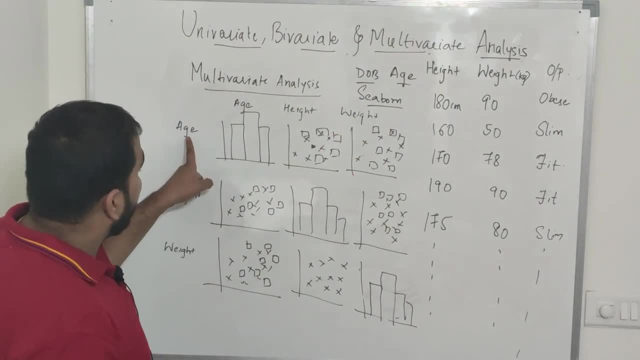 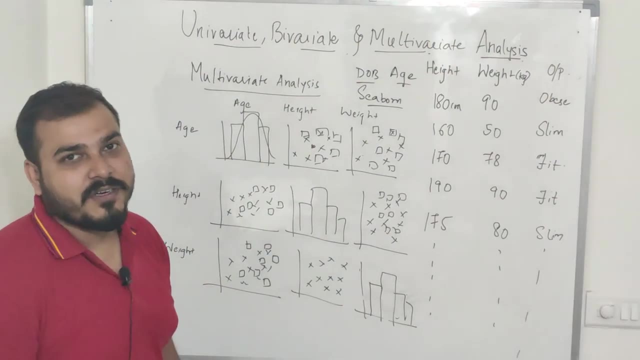 weight. now what will happen is that this diagram that will get plotted will be compared to this feature and this feature suppose, if i see age and age, definitely at that time i'll be getting a probability density function again. don't worry about histogram right now. in my upcoming classes, 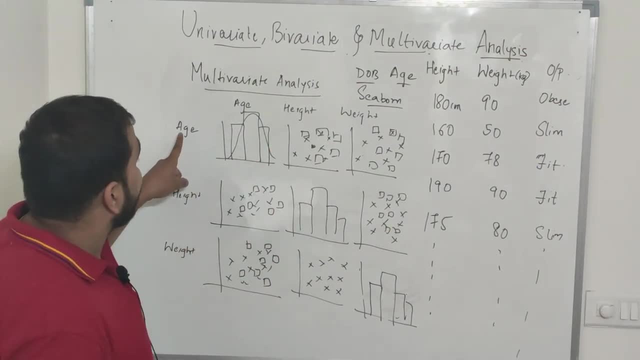 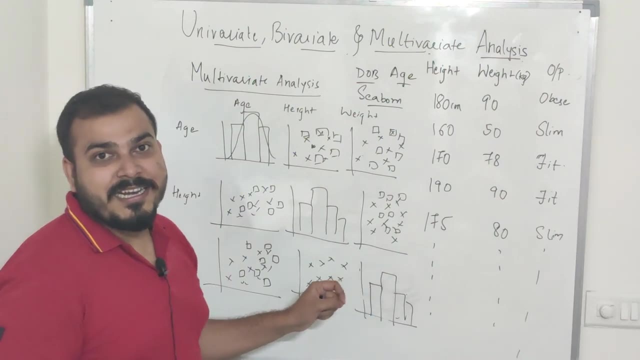 i'll be explaining you about that now. this particular diagram that i see is between age and height and based on that, that particular points are basically highlighted. similarly, this age and weight- you can see this points are getting highlighted in my next row when i go. this is: 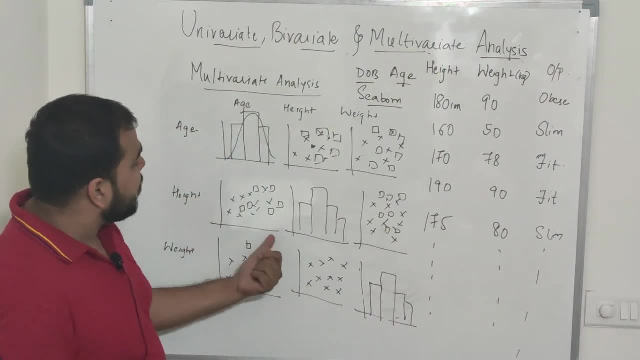 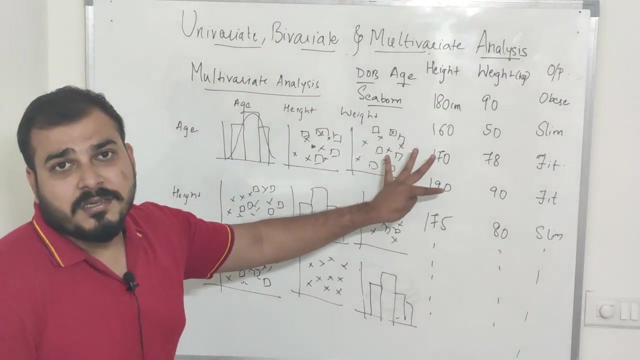 basically my height and this is basically my age. now i can see that, how this particular points has been plotted. all this will be explained in the part two and i'll be showing you practically how we can basically do with the help of seaborn with a perfect example. now understand this things, guys. this diagrams right? this diagrams can. 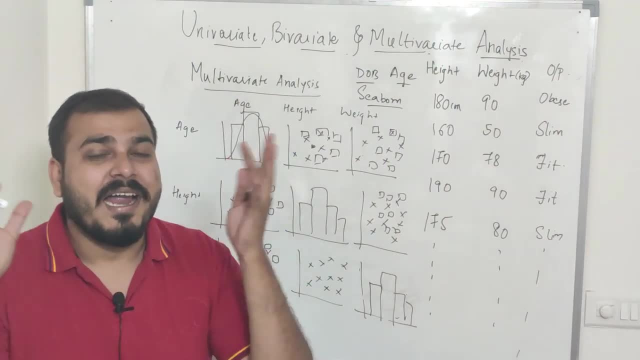 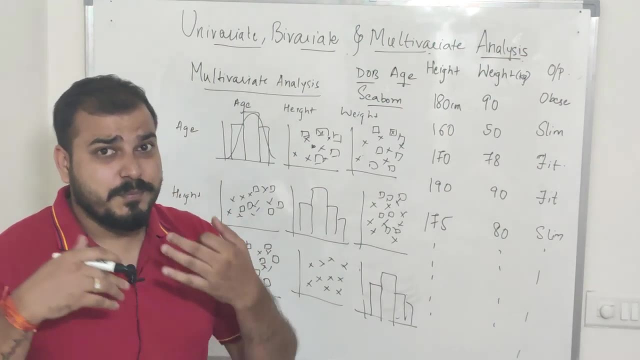 also lead to something called as correlation. you will get an idea of correlation. what does correlation basically mean? if you have not seen my videos in statistics, i have actually created a video on covariance pearson correlation. you can basically go and see that link. link will be given. 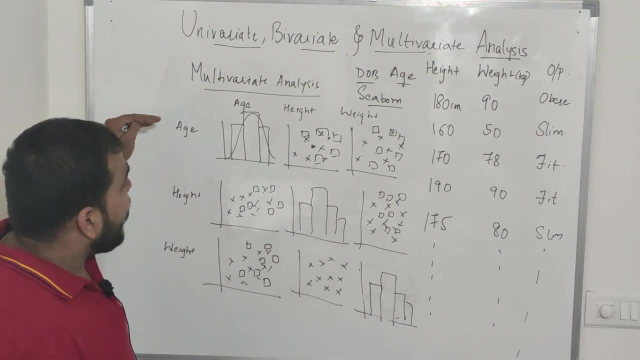 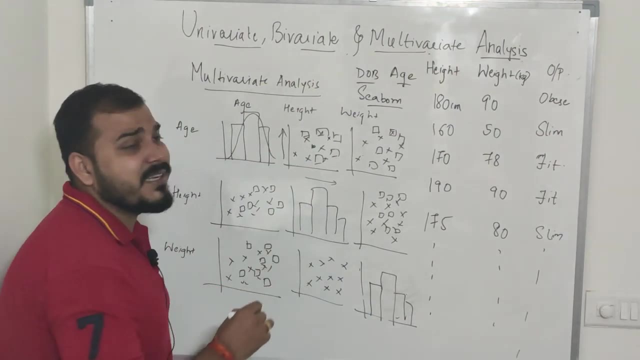 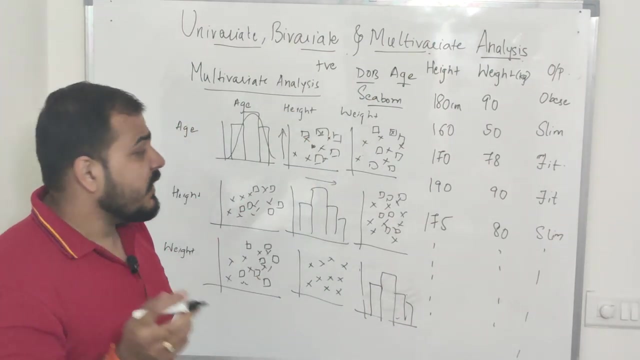 in the description. so what we can do is that whenever i see age and height, right, how does my age is increasing? can we find out whether the height is increasing? if it is in that way, then i'll basically get a positive correlation. okay, now the other thing is that if the age is increasing, whether 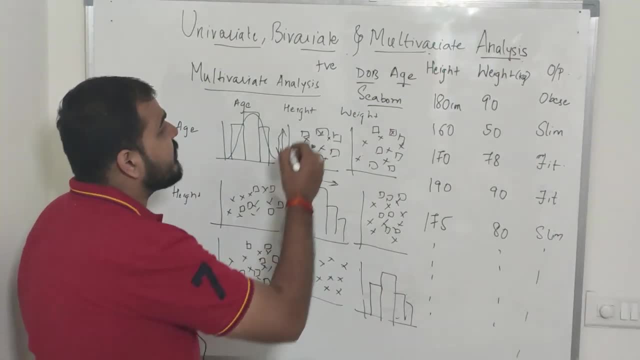 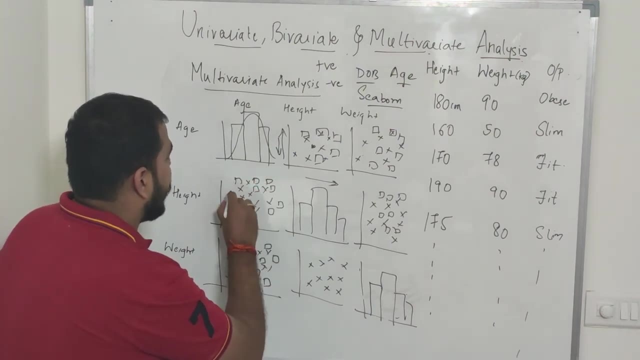 my height is decreasing. if this kind of scenario comes, then i will say that is my negative correlation. now there will be some points which will be evenly distributed, like this: okay, which will be evenly distributed, and i cannot come to a conclusion whether my age is increasing. that time my height? 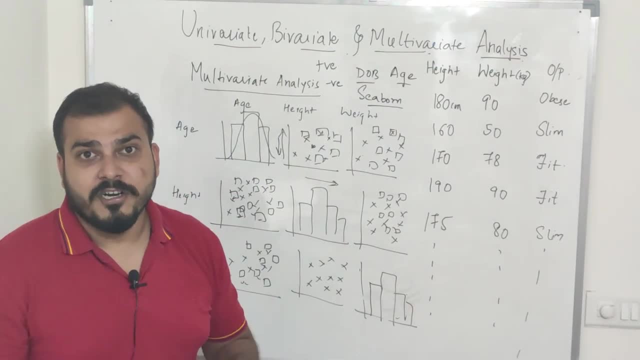 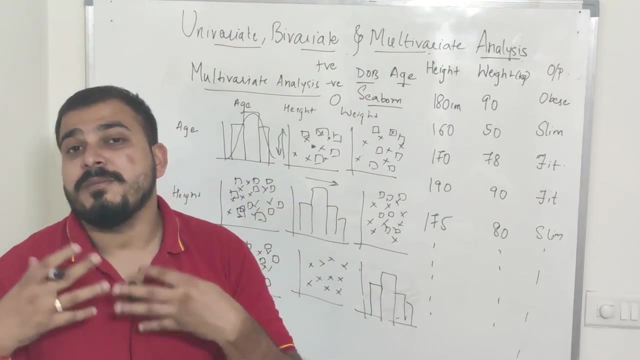 is decreasing, you cannot come to a conclusion for that case. at that time i will be saying that my correlation value is zero. okay, and this is what pearson correlation basically says. it helps us to find out the direction in which the features are basically going, whether one features increasing. 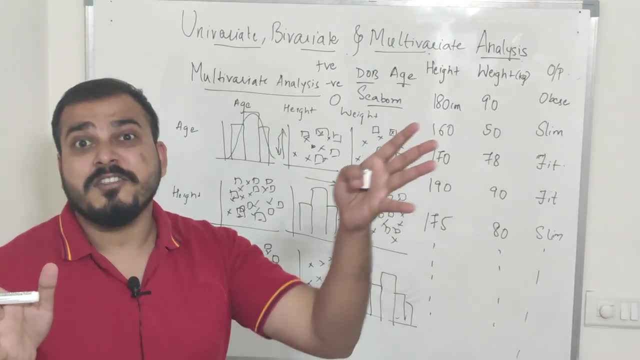 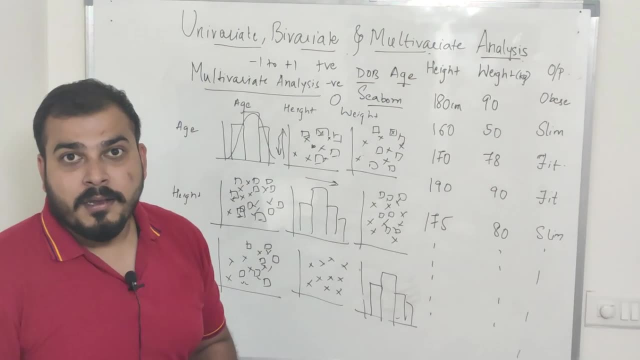 the other is also increasing, and always remember, the value will between between minus one to plus one, minus one to plus one, right, and this is pretty much important, guys, because with the help of this, it will help you to decide which is the best correlation between the two values. okay, so you can. 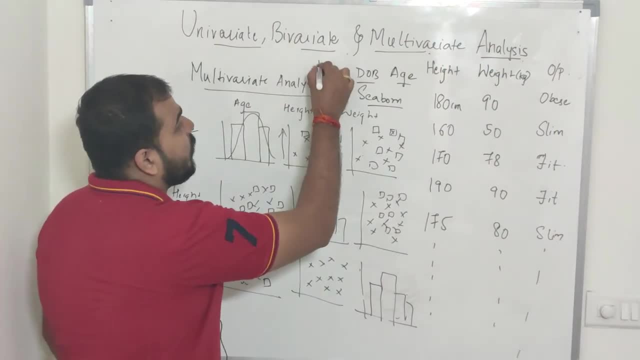 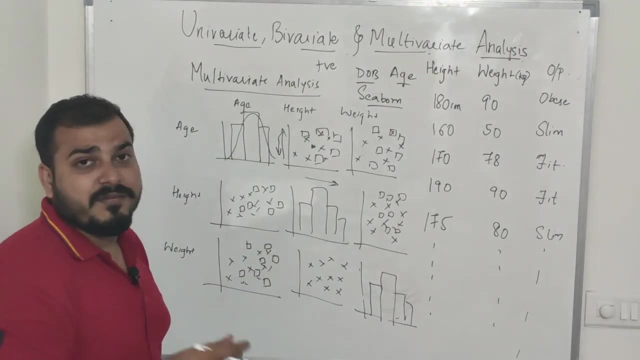 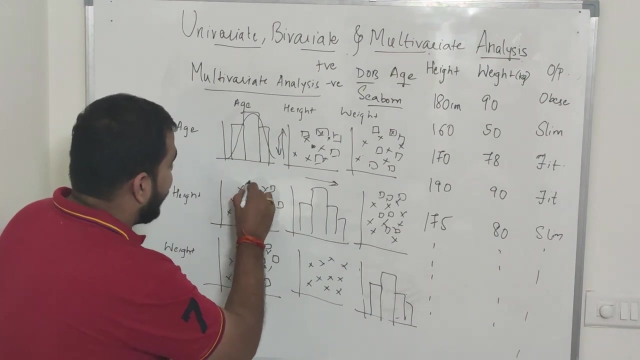 increasing. if it is in that way, then I will basically get a positive correlation. okay. now the other thing is that if the age is increasing, whether my height is decreasing, if this kind of scenario comes, then I will say that is my negative correlation. now there will be some points which should be evenly 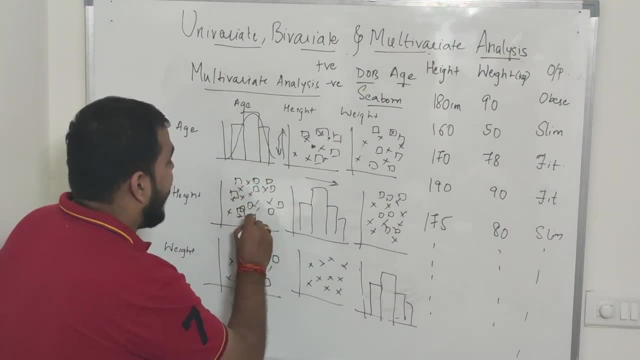 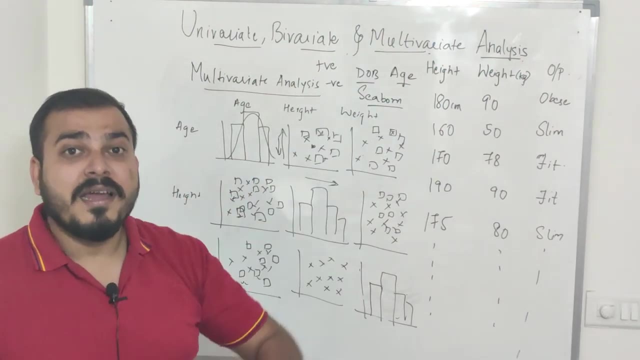 distributed like this, okay, which will be evenly distributed. and I cannot come to a conclusion. whether my age is increasing that time my height is increasing, whether my age is increasing, that time my height is decreasing, you cannot come to a conclusion for that case. at that time I will be saying that: 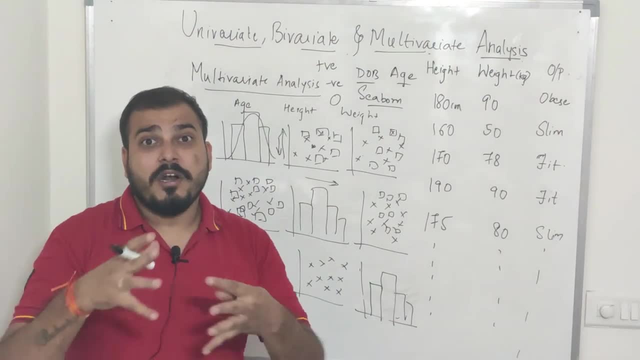 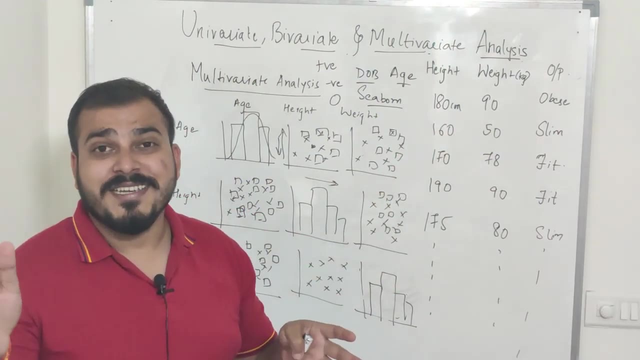 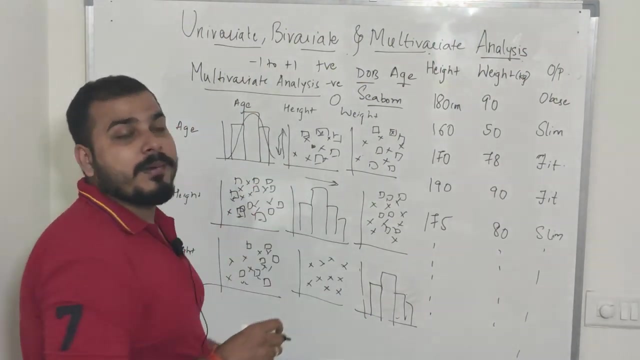 my correlation value is zero. okay, and this is what Pearson correlation basically says. it helps us to find out the direction in which the features are basically going. whether one feature is increasing, the other is also increasing. and always remember the value will between between minus one, two plus one. minus one, two plus one, right, and this is 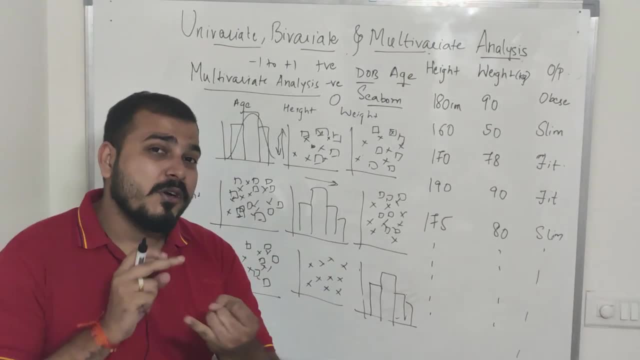 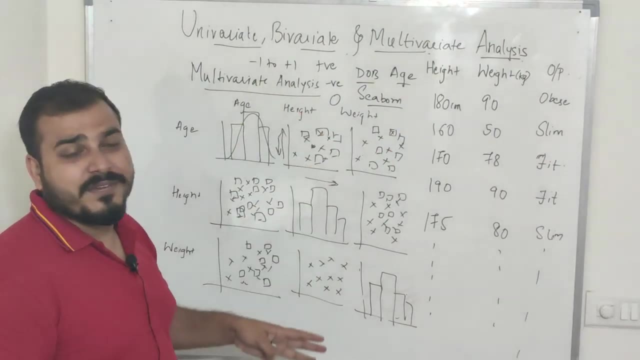 pretty much important, guys, because with the help of this it will help you to decide which algorithm you can go ahead with. because I understand over here if I'm having a positive correlation. if I see this particular classification problem, can I just draw a straight line and basically divide those point. so, or? 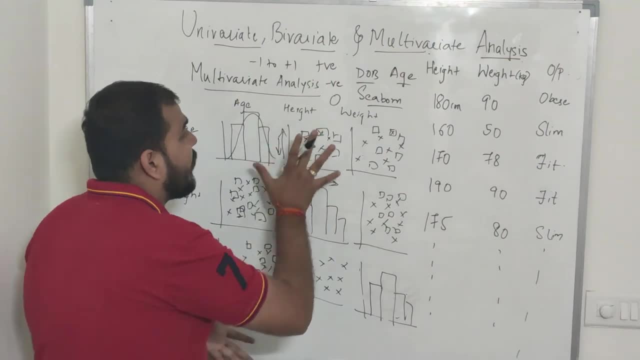 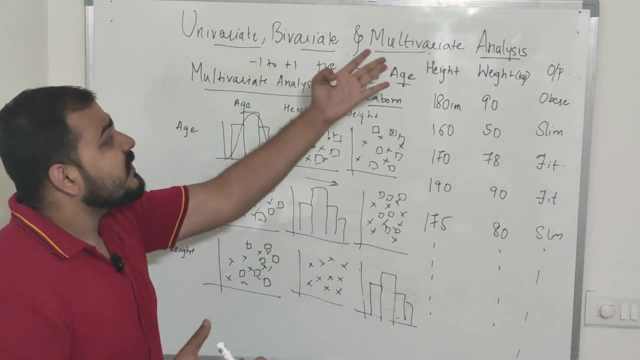 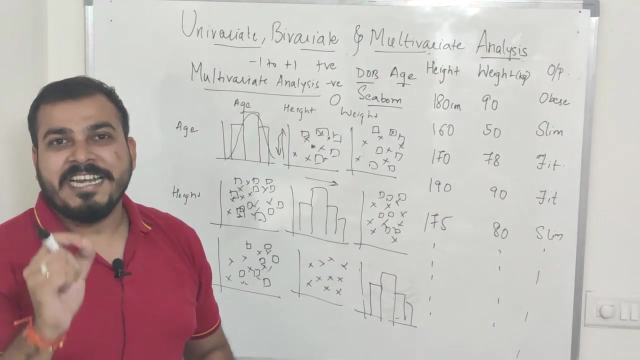 should I use some non-linear classifying problems to basically apply this particular problem to this particular problem statement? so all this information can be took out from this and this is what is basically a univariate and bivariate and multivariate analysis. this is the fundamental step in exploratory data analysis and always remember, guys, this. 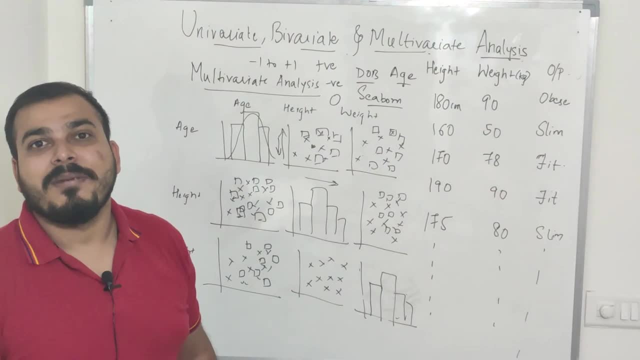 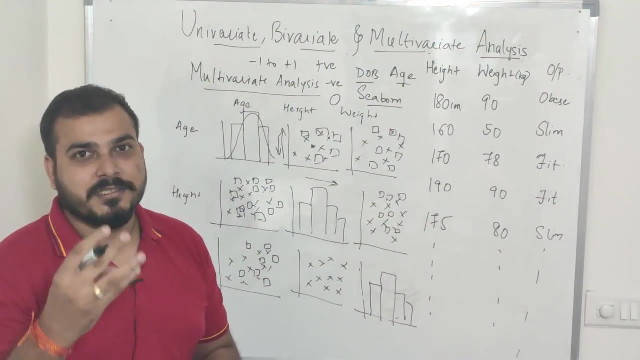 is my part one. in my part two i'll also be showing you the practical application by considering this kind of example. there i'll be taking an example of irish data set and then i'll show you. there are four features as petal length, sepal length, petal width and sepal. 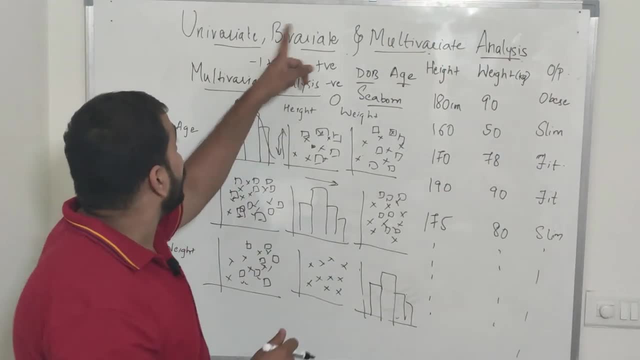 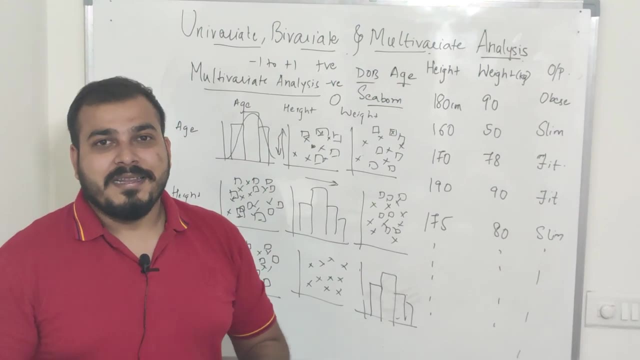 width. first of all i'll go and do a univariate analysis, then i'll go and do a bivariate analysis, then finally i'll go and do a multivariate analysis and try to show up that particular problem with you. at that time you will understand more things about that, understand this pair plot. 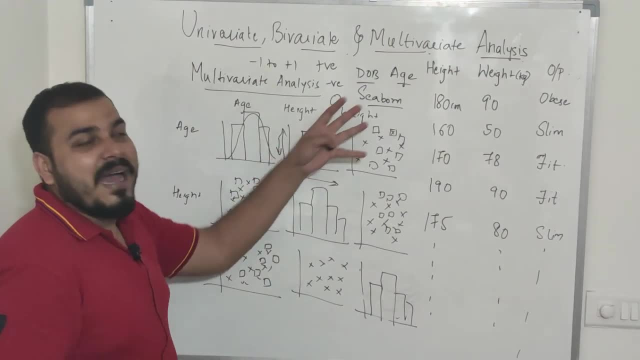 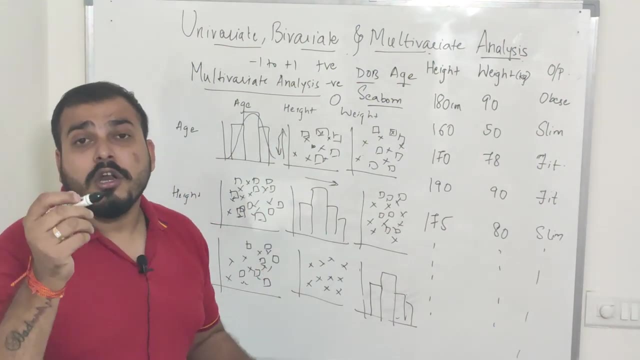 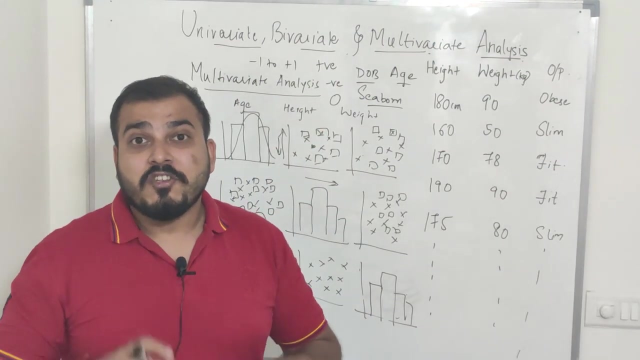 which algorithm you can go ahead with. because, understand over here, if i'm having a positive correlation, if i see this particular classification problem, can i just draw a straight line and basically divide those points? so or should i use some non-linear classifying problems to basically apply this particular problem to this particular problem statement? so all. 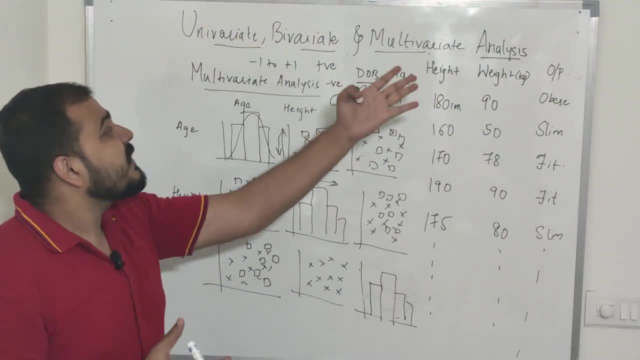 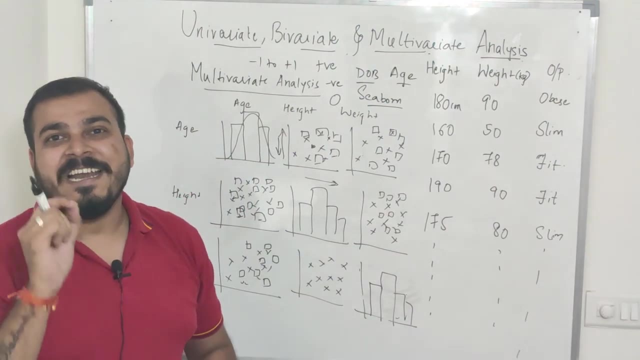 this information can be took out from this and this is what is basically a univariate and bivariate and multivariate analysis. this is the fundamental step in exploratory data analysis. and always remember, guys, this is my part one. in my part two i'll also be showing. 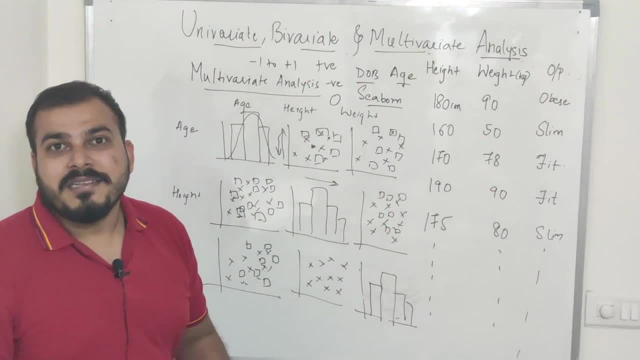 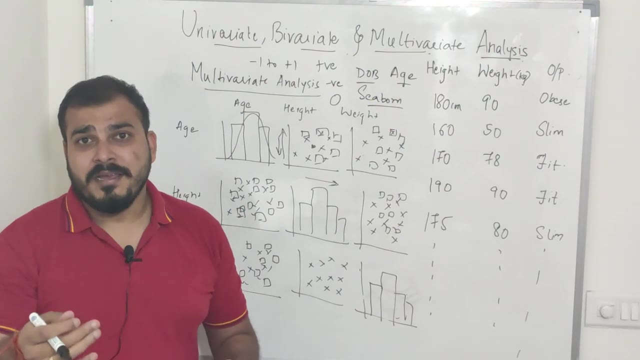 you the practical application by considering this kind of example. there i'll be taking an example of irish data set and then i'll show you there are four features as petal length, sepal length, petal width and sepal width. first of all i'll go and do a univariate analysis. then 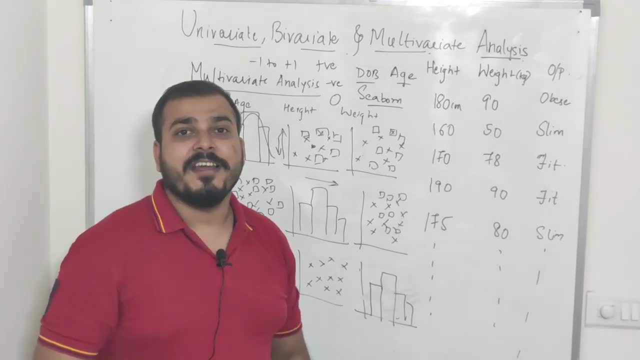 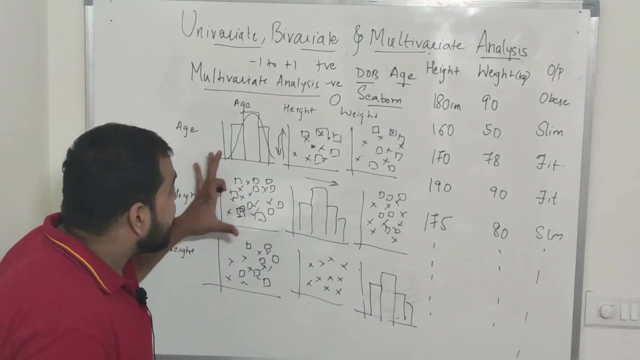 i'll go and do a bivariate analysis. then finally, i'll go and do a multivariate analysis and try to show up that particular problem with you. at that time you will understand more things about that. understand this pair plot also. understand this pair plot also. understand this pair plot also. 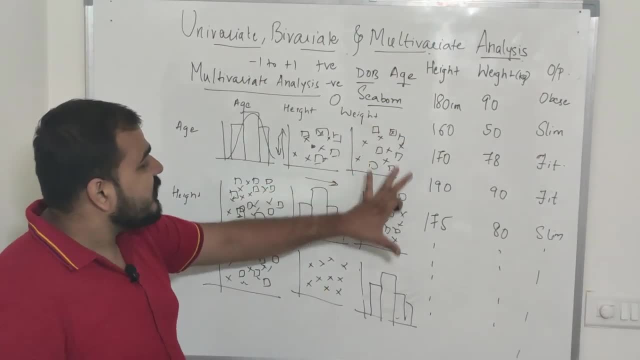 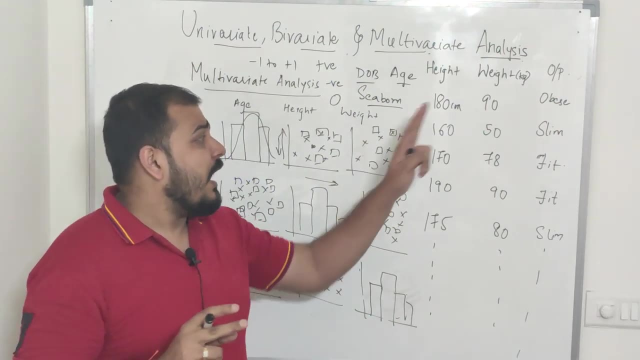 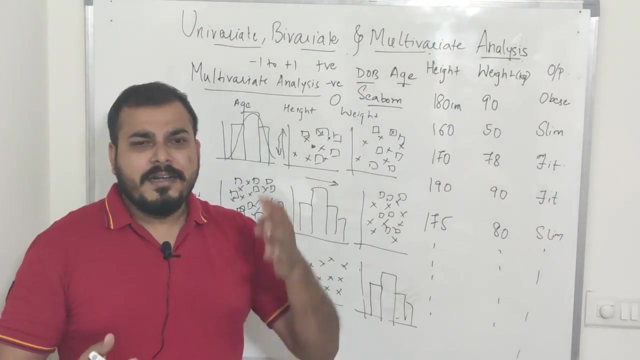 then if i am actually finding the correlation also with respect to this particular value only, i'll be either getting positive, negative or zeros value right if two features are more correlated with respect to the output, right. both the features are basically important, you know, and suppose if both the feature are 90 correlated i can drop one of the feature because both both of them features. 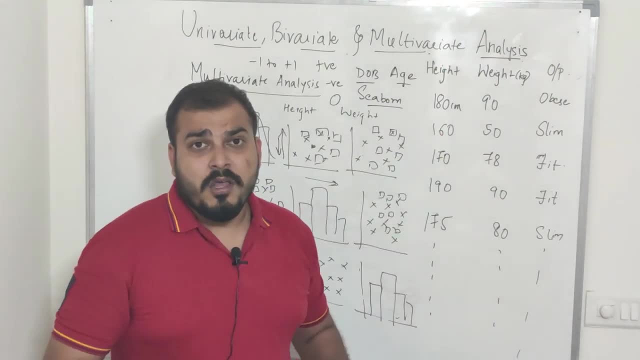 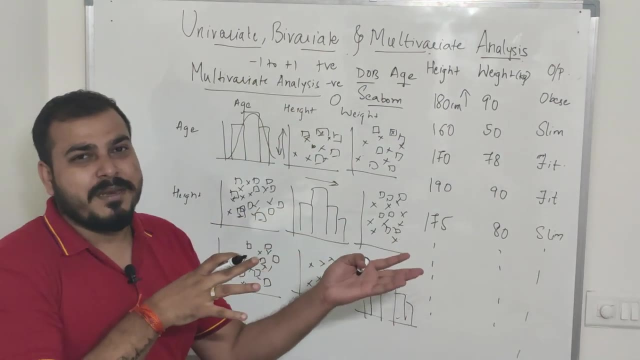 are basically similar, right, similar with respect to one output. always remember, guys. again let me repeat what did i mean? suppose my height is increasing and my suppose this is. this is basically my output as a classifier problem. but if i had an output of regression, problem, okay. and if 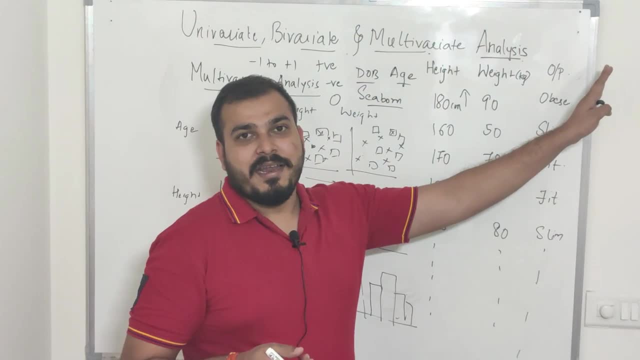 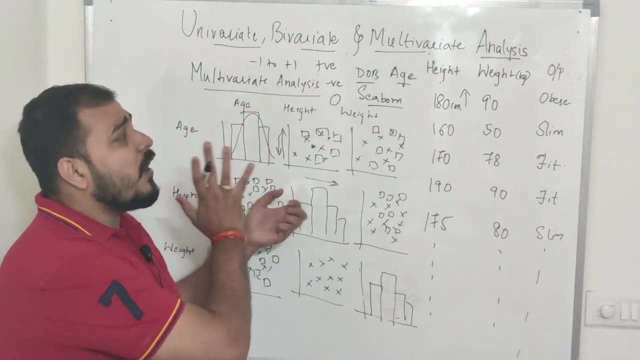 i suggested when my height was increased. this value is also increasing right at that time. i can say that this height is basically correlated with the output. all this kind of information can be gained from this analysis and this is again the fundamental step in exploratory data analysis. so i hope you. 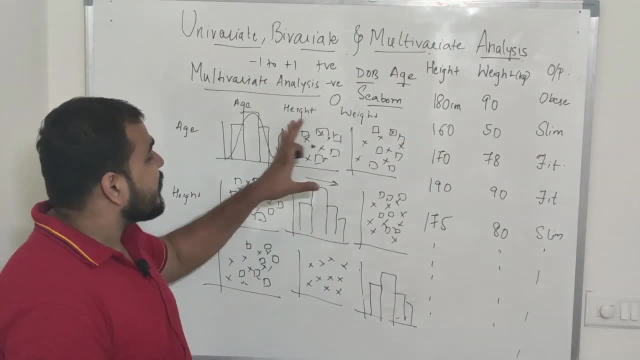 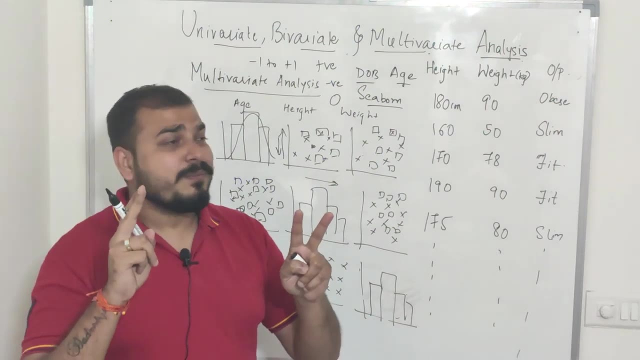 also, then if i am actually finding the correlation also with respect to this particular value only, i'll be either getting positive, negative or zeros value right. if two features are more correlated with respect to the output, right? both the features are basically important, you know, and suppose if 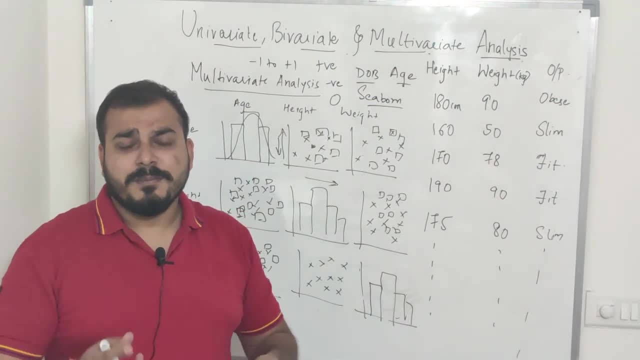 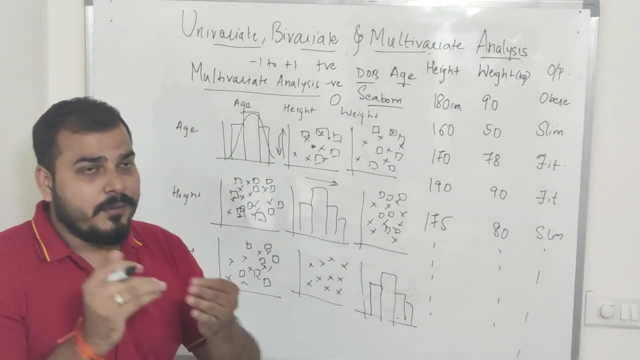 both the feature are 90 correlated. i can drop one of the feature because both both of them features are basically similar. right, similar with respect to one output. always remember, guys. again let me repeat what did i mean? suppose my height is increasing and my suppose this? this is basically. 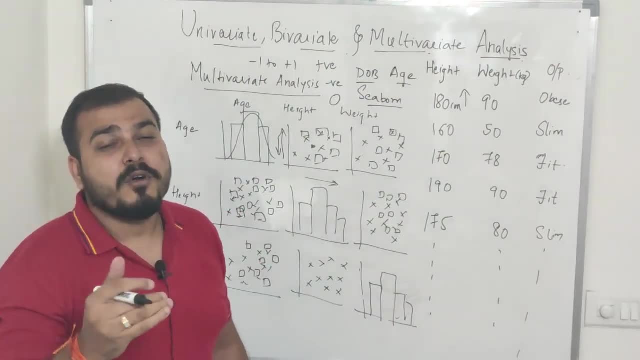 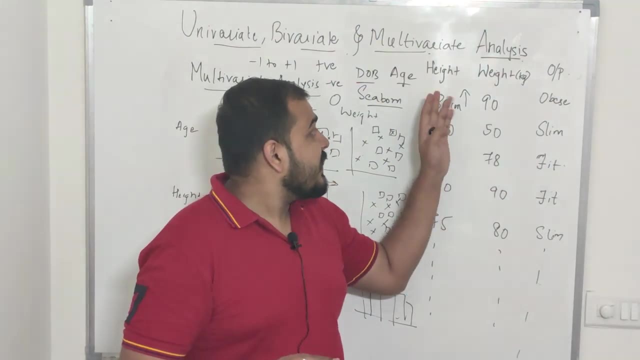 my output as a classifier problem. but if i had an output of regression, problem okay, and if i suggested when my height was increased, this value is also increasing right at that time, i can say that this height is basically correlated with the output. all this kind of information can be gained. 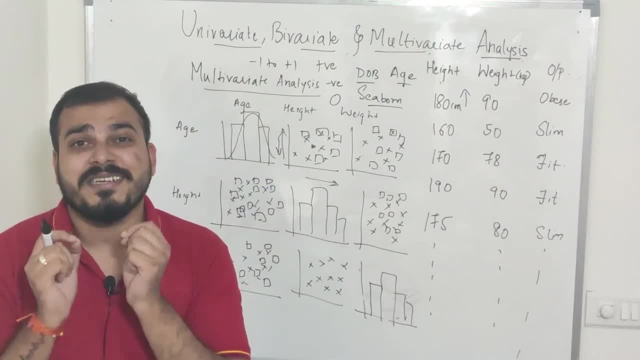 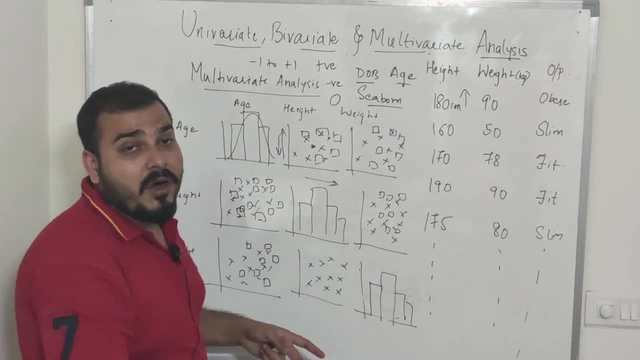 from this analysis and this is again the fundamental step in exploratory data analysis. so i hope you understood this particular video. i hope you understood whole this, all these things, why we cannot drop 4d plot. you know, because of the 4d plot i can basically do a multivariate analysis and because of this, when i do a multivariate, 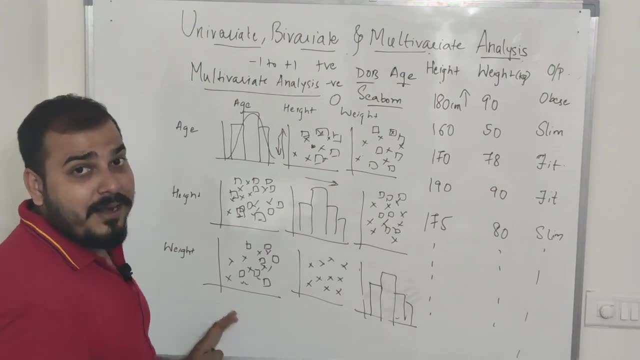 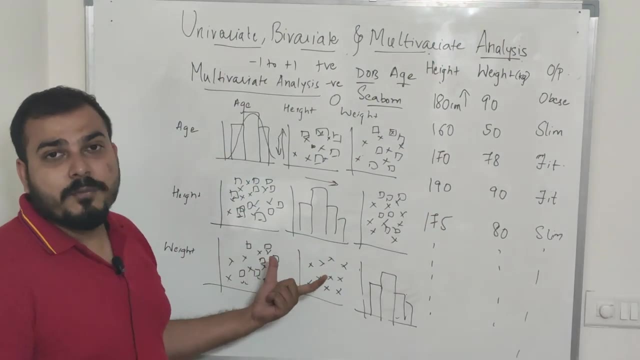 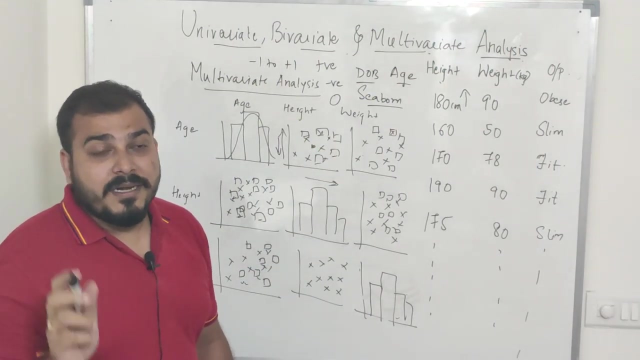 analysis. this is how it is basically done. all the features will be populated. and remember, guys, over here category features will not come, only integer continuous values will be able. you'll be able to plot over here. you will not be able to plot category feature. yes, you can classify with the help of category, category feature okay, but you cannot plot a. 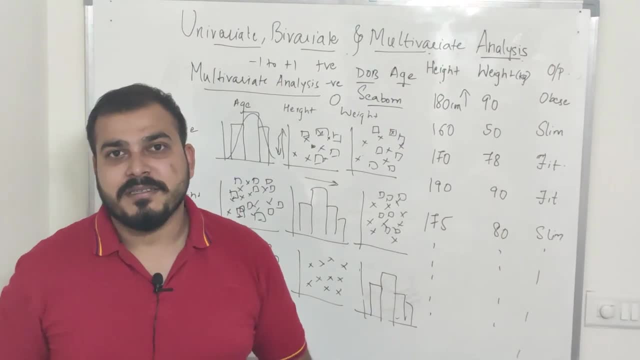 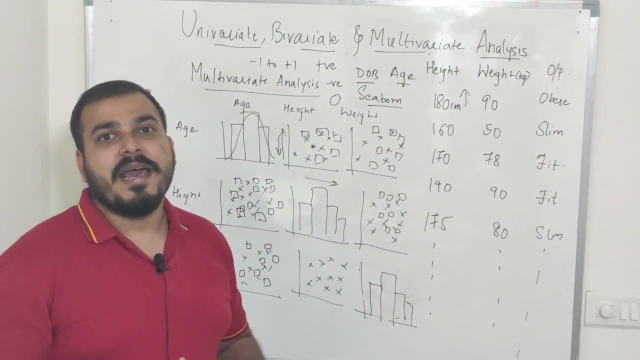 category feature, because you know, category features are fixed number of occurrences. right, they have fixed number of occurrences, but in continuous values you have some numbers and numbers are only used for using the plotting the diagrams like this. so i hope you understood this particular video. please do subscribe the channel if you have not. 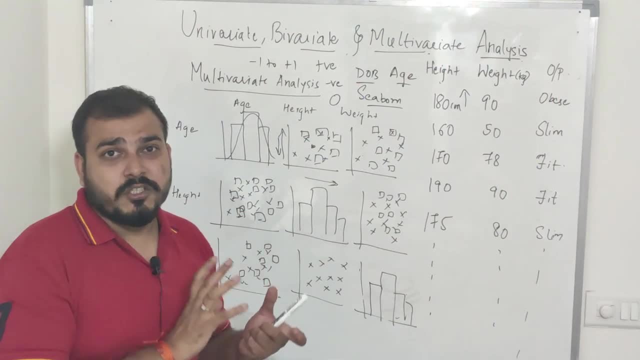 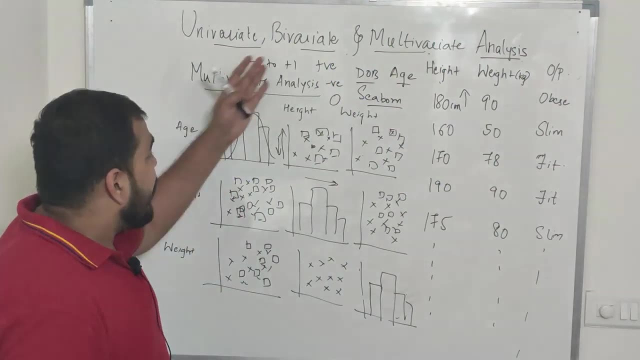 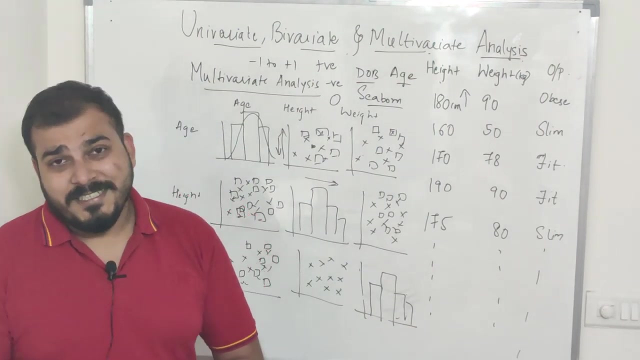 already subscribed. in the next video, i'll be coming up with a concept called as histogram- probability density function- cumulative density function- and then i'll also go with the practical application and show you, implement all these things in front of you. and this is all the part of statistics, exploratory data analysis, right? so yes, why i'm saying statistics? because 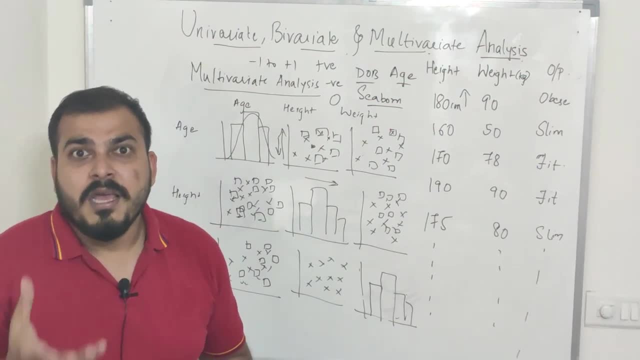 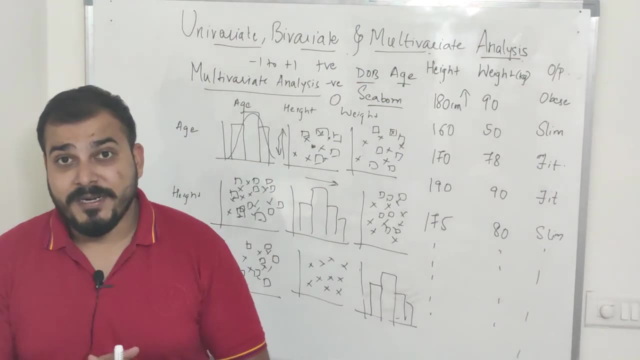 probability density function, when i'm explaining some concepts of statistics will come. when i'm explaining cumulative density function, again some concepts of statistics and maths will come. so yes, this was all about this particular video. please do subscribe the channel if you have not already subscribed. i'll see you all in the next video. have a great day. thank you, one doll. 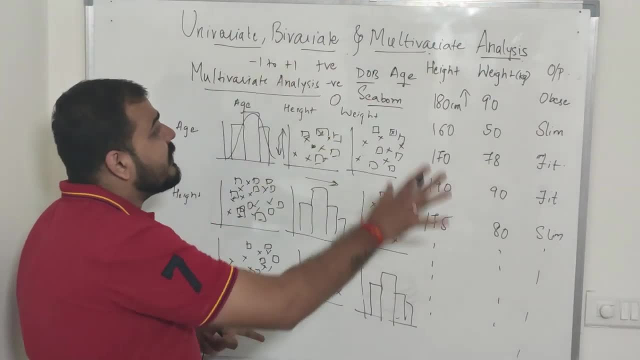 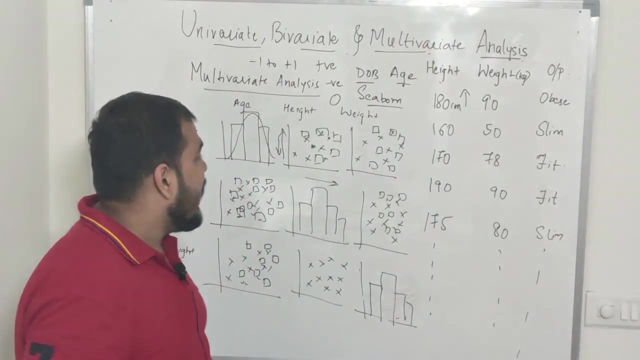 you understood this particular video. i hope you understood whole this, all these things, why we cannot do a 4d plot. you know, because of the 4d plot, i can basically do a multivariate analysis and because of this, when i do a multivariate analysis, this is how it is basically done.